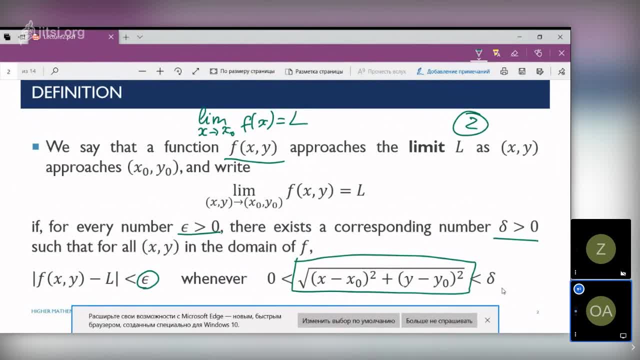 And this expression should be between zero and delta. We tried to learn, we tried to understand this with the function of single variable when we studied higher mathematics, one course. But now it's just expanded with the second variable, which is y. It's almost similar, almost same, except we have y here and we. 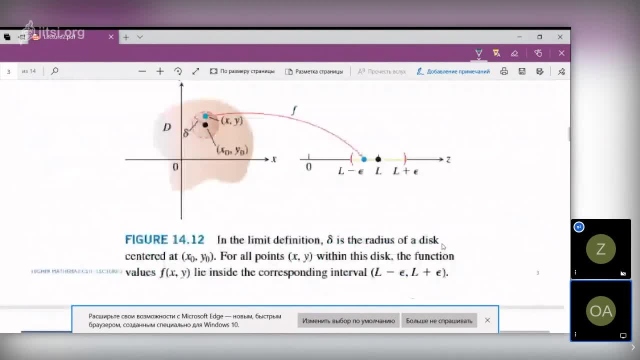 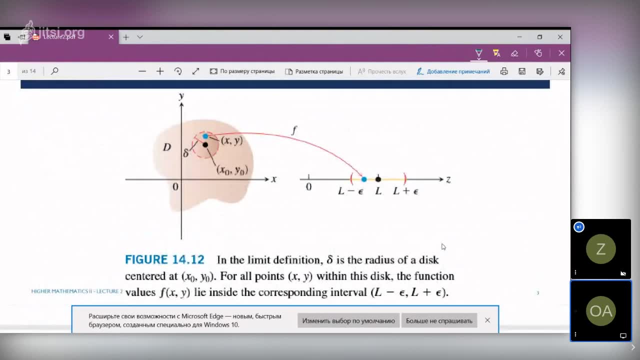 have y here also In this figure we can check this one. In the function of single variables, the x, we had just x and we took x from the number line. like this one, it was x and we took any number x. 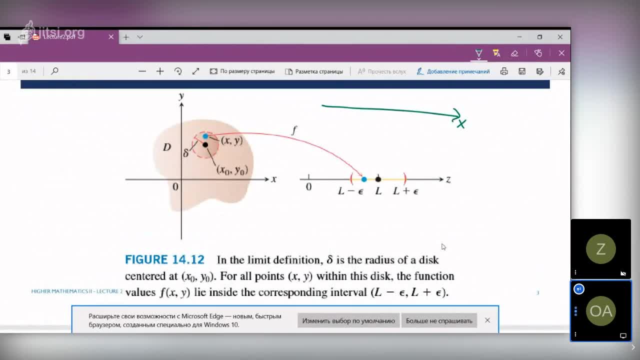 But when we are approaching functions of several variables, for example two variables, we have a region this kind of- we learned this in the first lecture- we have a region, So we have a region. So we have a region this kind of- we learned this in the first lecture- we have a region. 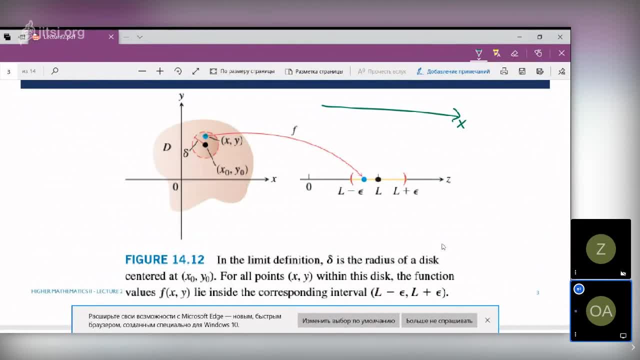 So we have a region, And this is the point, x and y, If I take for the function of single variable- here x1, and then for the function of double variables with two variables. I can choose a point from this coordinate plane, from the. 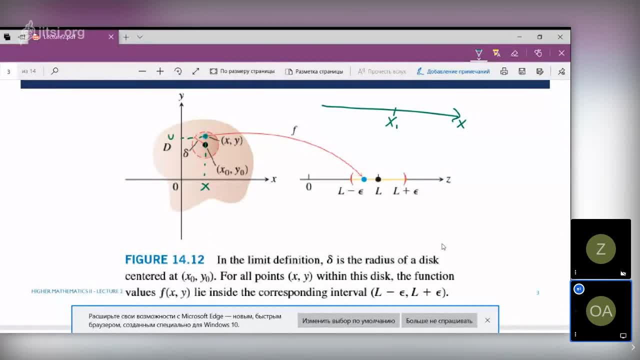 coordinate plane. So it will have its x and it will have its y. So this is the point, And this point should approach to the x0, y0, which is this black line, This blue point should approach to the black point. 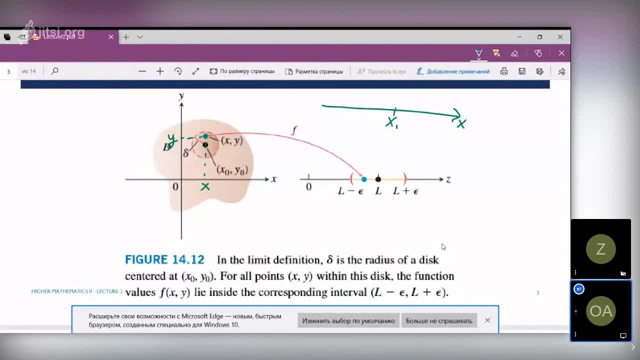 And when it's approached in this delta radius, the value of function should approach to the number l. The value of function will have to choose from this number line, Because it doesn't matter if function has one variable, two, three or etc. 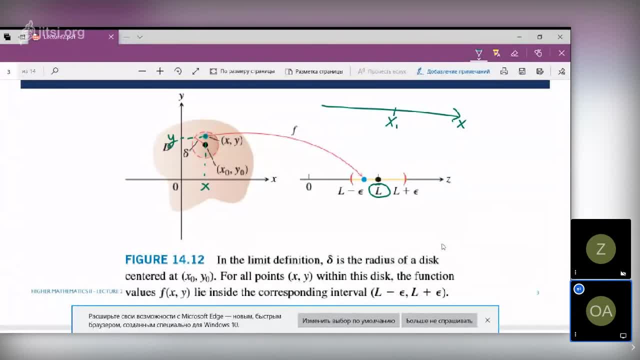 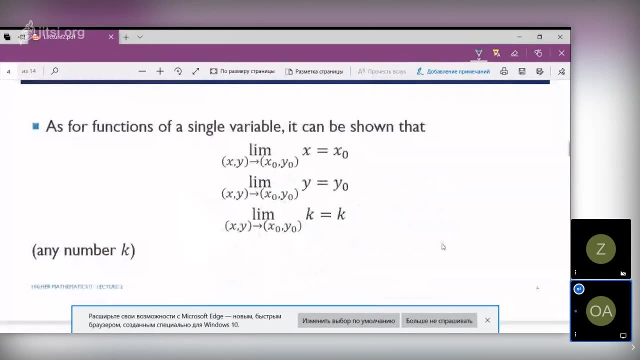 But the value of function will be a number, Any kind of number. So this number should approach to number l. So this is the formal definition of function of double variable, For example, as for functions of single variable, it can be shown that limit x and y when x and 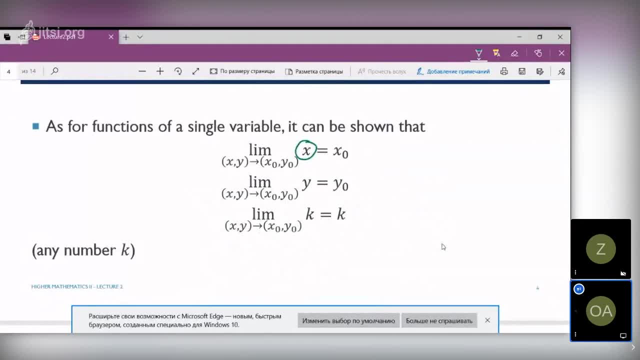 y approach to x0, y0.. So here it's x. What is this? This is our function. So it says: Now we have f of x. y equals to x. This is our function. Function is just x. 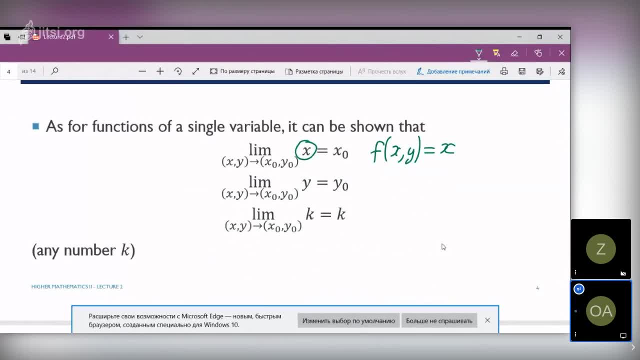 We don't have y. So if we have the function x, it says: put instead of x, x0.. Put instead of y: y0.. So I just have x here. Instead of x, I put x0.. 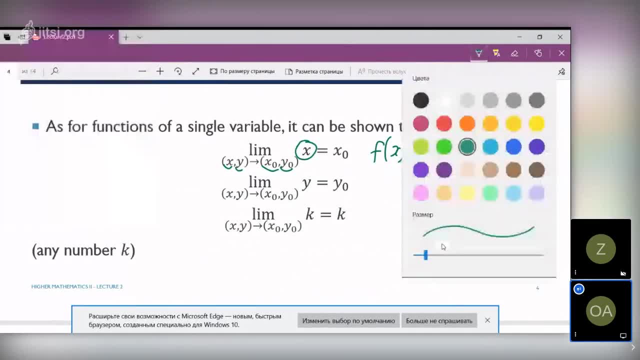 So I got the answer x0.. So this is the answer x0.. In the second case, limit x and y approach to x0, y0. Our function now f of x, y is y. We don't have x in this case. 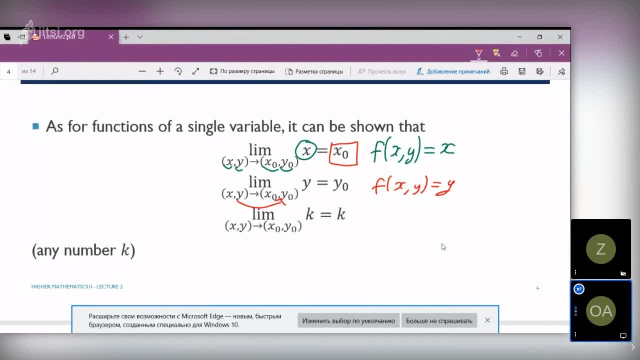 So just put instead of y y0. So the answer is y0.. In the third case we have here limit x, y tends to x0, y0. And the function is k. f of x, y equals to k. 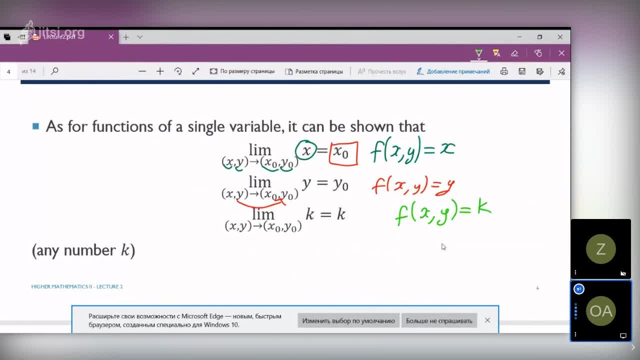 k is any constant number. So if you look carefully here, we don't have x, We don't have y in the function, So the answer remains the same as k. When we started to learn functions of single variable and we tried to find their limit, 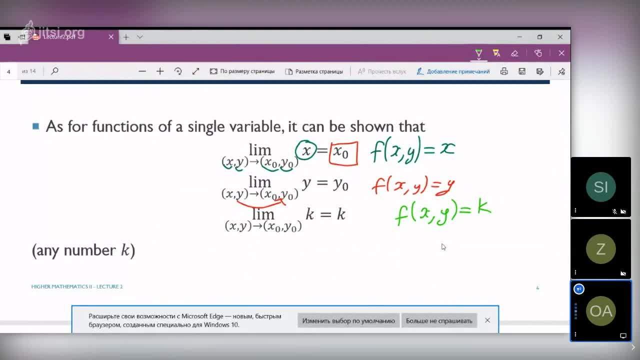 when the function is any number, any constant number. we had similar examples. We tried to solve it. For example, limit x tends to like 7. But the function is 13.. What is the answer for this one? Can you see this green text? 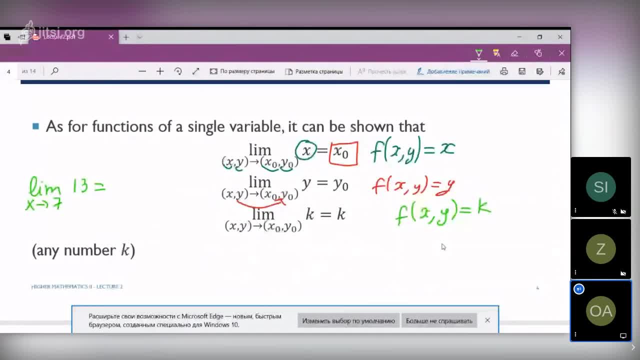 Green expression here. Yes, yes. What is the answer for this one? Limit x tends to 7.. The function is 13.. The previous course: higher mathematics one. So what is the answer? 20? Yes, 13.. 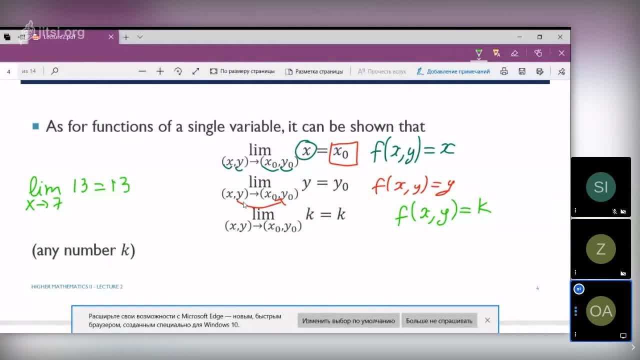 It's 13.. No, it's 13.. That's right, Our function is 13.. But it says: if f of x could say: do we have x here? Do we have x? No, we don't have x here. 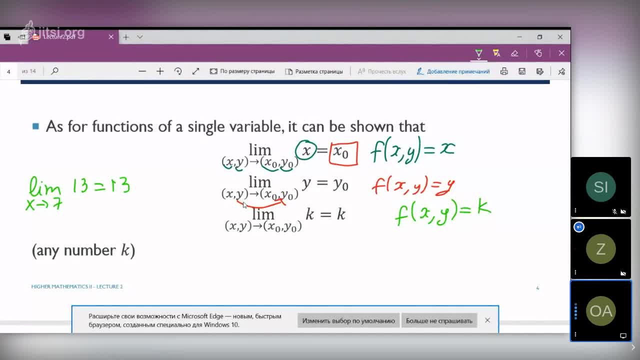 So the answer will be 13.. This one is also similar. For example, I can write one more example: Limit z tends to z0.. The function is 13x. What is the answer? The function is 13.. 13, or only x? 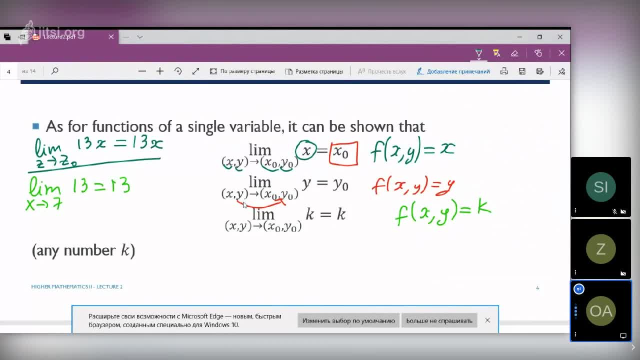 13x, 13x, 13x. yes, This question says that instead of z, put z0.. Instead of z, put z0.. But do we have z here? No, we don't have. So the answer will be this expression: 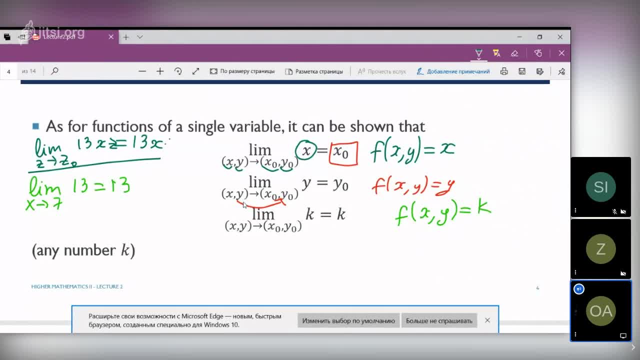 We had z here, for example x, z, It will be x z 0, if we had, but we didn't have it first of all, so it was 13x With the functions of several variables, like double variable, like this one, x and y- or triple variables, x, y, z or other functions. 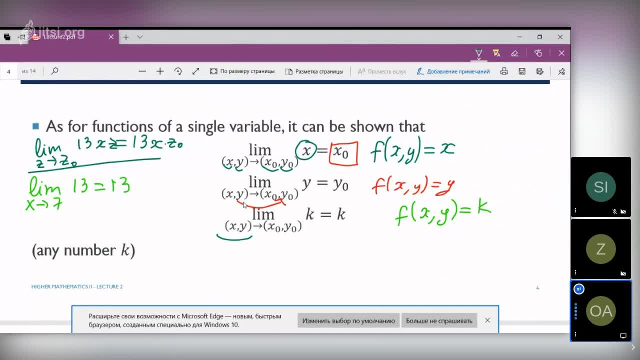 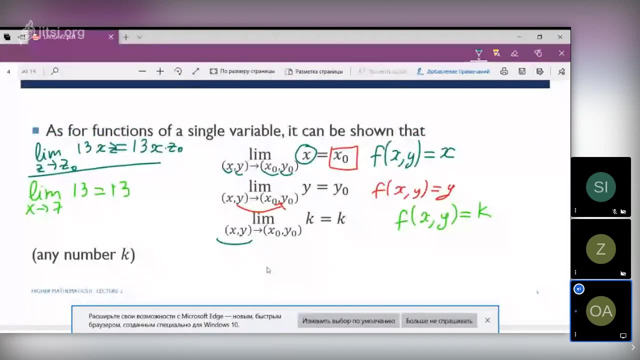 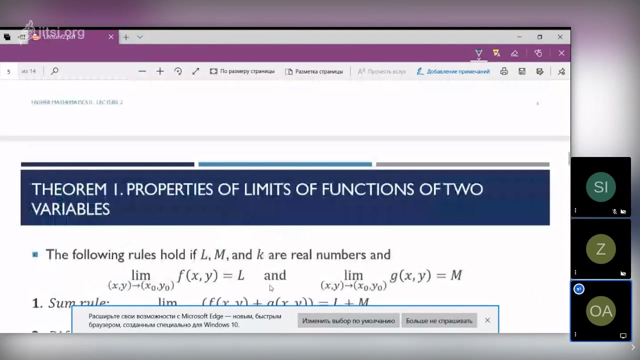 these rules are acceptable. It will remain the same, the similar rules. Just we have one molar, but we have two molars. If we have an x and y, it's also same. So here the rules about the calculating limits. 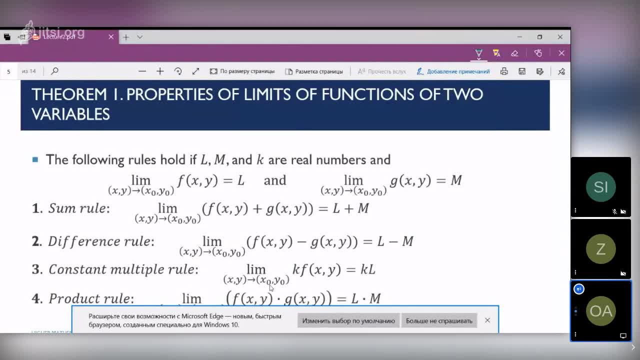 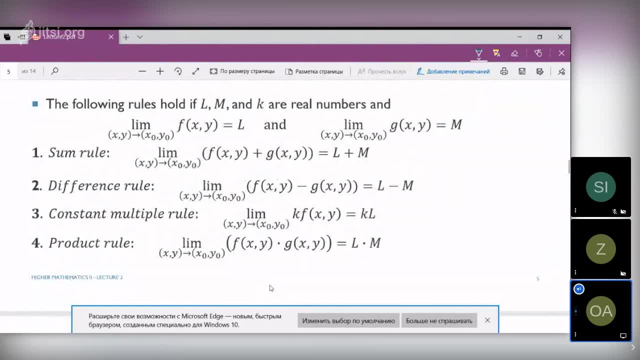 The theorem 1.. Properties of limits of functions of two variables. The following rules hold if L, M and K are real numbers, L, M and K are real numbers And the limit of f when xy tends to x0, y0 is L. 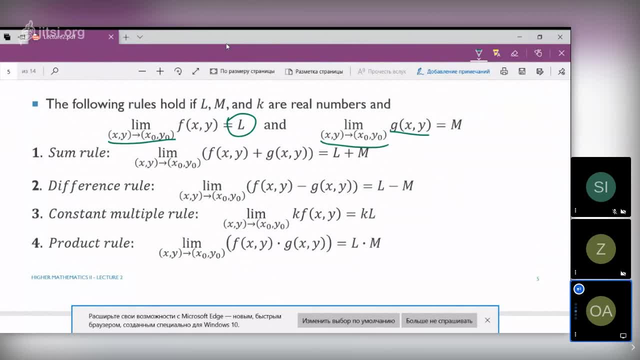 And the limit of g when xy tends to x0, y0 is M. We had this rule. There were seven rules in the previous course on mathematics. 1 for the function of a single variable. Now we're extending this rule for the function of double variables. 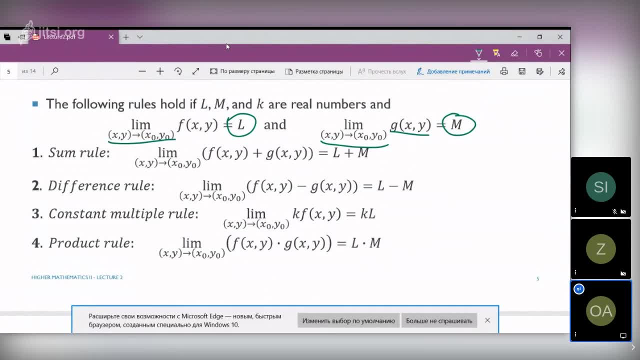 For the function of two variables. For example the first rule, sum rule. it says limit xy tends to x0, y0. And in the penalty list we have f of xy plus g of xy. So how to calculate this? 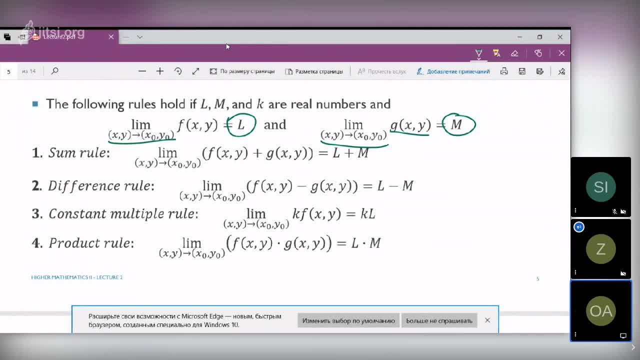 We calculate the limit of the sum, We need to know the each limit. So what is the limit of f of xy, when xy tends to x0, y0?? So first of all we have to find the limit of this one. What is the limit of this one when xy tends to x0, y0?? 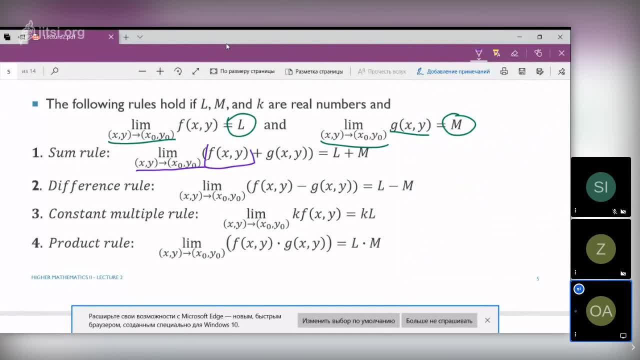 We know this. It's L. It's given Limit x, It's L. So we wrote here L, Then plus. What is the limit of this? one Second expression: When xy tends to x0, y0?? It's M. 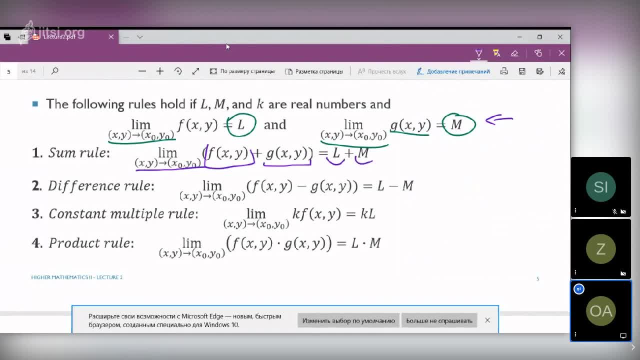 It's given here. So plus M. So this is the answer. For example, if I have the limit, xy tends to: Okay, not the x0, y0.. Let me write it here: Okay, 2 and 3.. 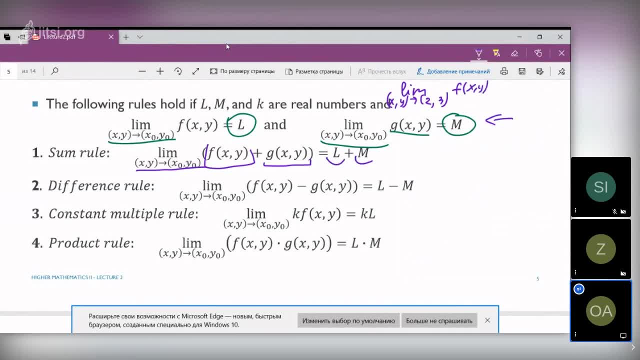 And I have some functions here, For example f of xy, It's a sign of function, And if this is equal to 7.. And if I have another one, Let me write here: Limit xy tends to 3.. 2 and 3.. 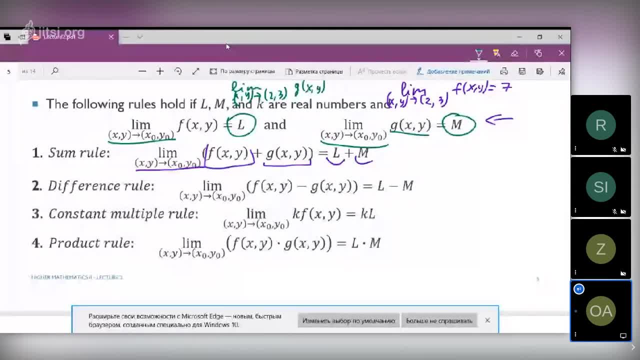 g of xy equals 3.. Okay, This expression. The first rule says limit xy tends to x0.. Sorry, Not x0.. Now it is now 2 and 3.. 2 and 3.. f of xy plus g of xy will be 3 plus 7.. 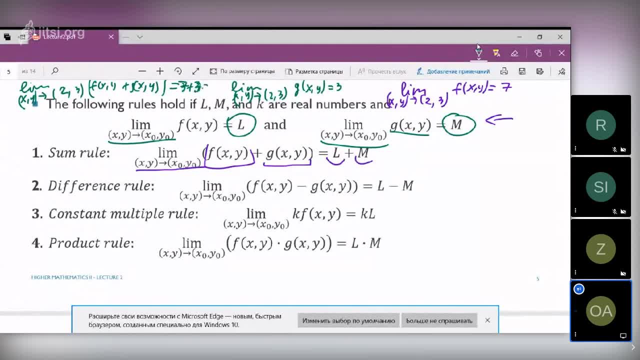 7 plus 3.. 7 plus 3.. And it will be 10.. Yeah, The rule says about this one, The sum rule. Yeah, Next one is the difference rule, Difference rule. It's almost similar, But we have, instead of plus, the minus sign. 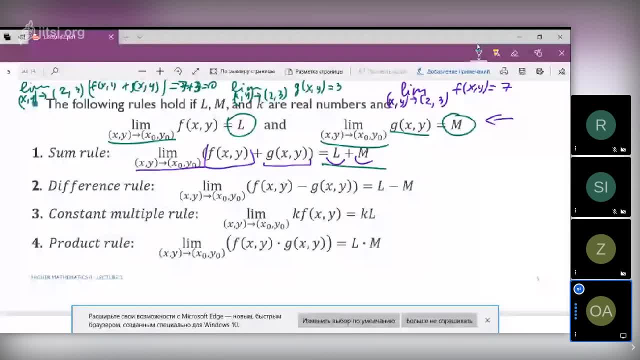 Yes, Destruction Minus sign. You know already what is the f of xy's limit when xy tends to x0, y0.. It's L And it's xy, And it's y, And it's y And it's y. 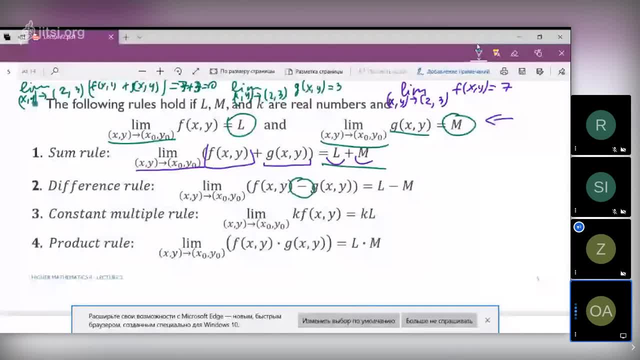 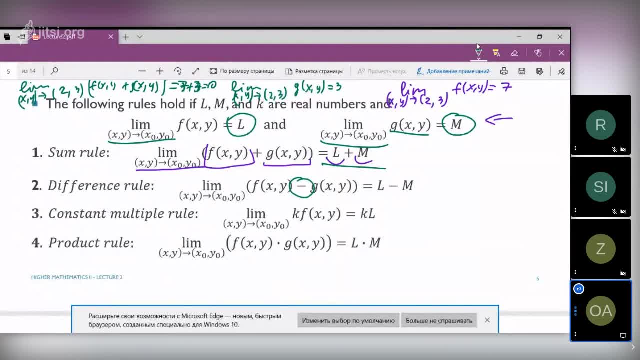 And xy tends to x0, y0.. and xy tends to x0, y0.. It's L and we also know the limit of g of xy. It's xy tends to x0, y0.. When xy tends to x0, 0.. 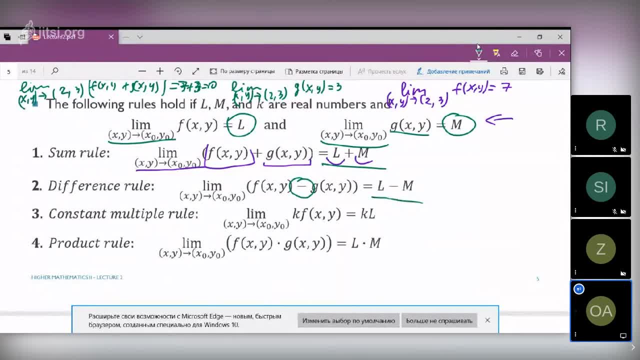 It's M, So the answer will be L minus M, This one, And here we have the constant multiple. Constant multiple. The question says the limit xy tends to the social and what we've done We need at xy tends to x0, y0.. 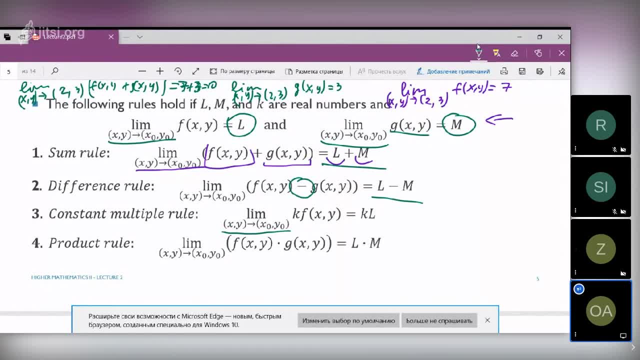 have a function: k times f of x y. so it's k times f of x y. so we have your k itself. when calculating this, first of all we have to add k, because it's a constant number, and times f of x y. the limit is l. 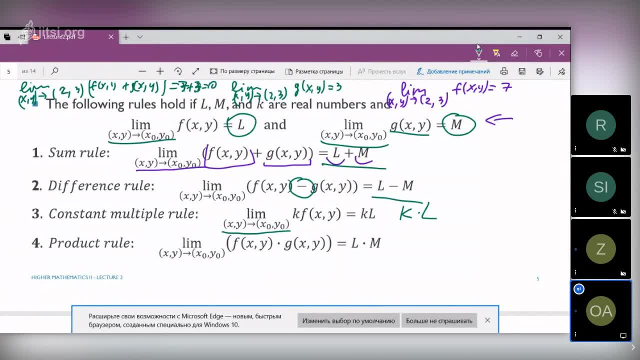 so, first of all, we have to write the constant number and times the limit. and one more rule which is productive, productive, we need a product: f times g, when x, y tends to x, zero. y zero is l times m, l times n, because f of x, y is, in our case. 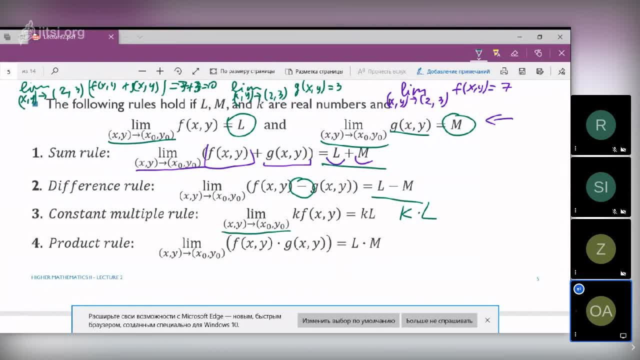 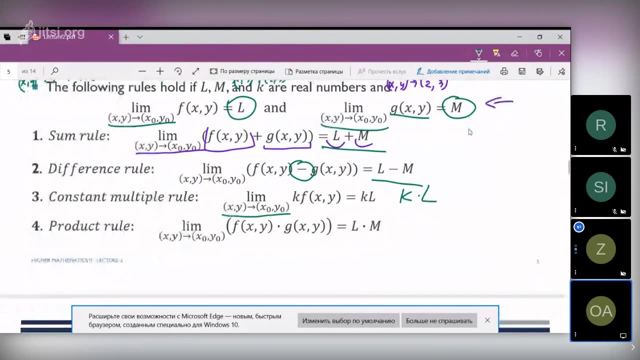 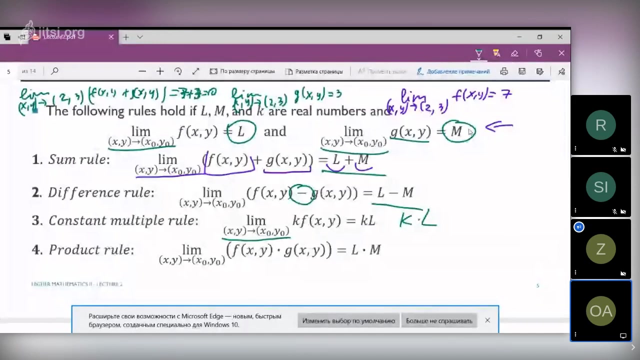 limit is l and g of x. y's limit is m, so the answer will be l times m. in this case, can you give an example for the third third rule: constant, multiple rule. can you give an example for this? for the third one: constant, multiple, constant, multiple. okay, for example, we have a limit. 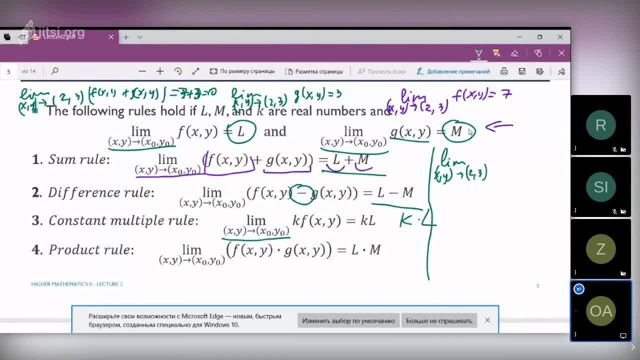 x, y tends to two and three and function i. i think it's better to write x squared times y. so can you calculate this? limit, this one on the right side, dark green: x tends to two and three and function y tends to two and three, x tends to number two, y tends to number three. 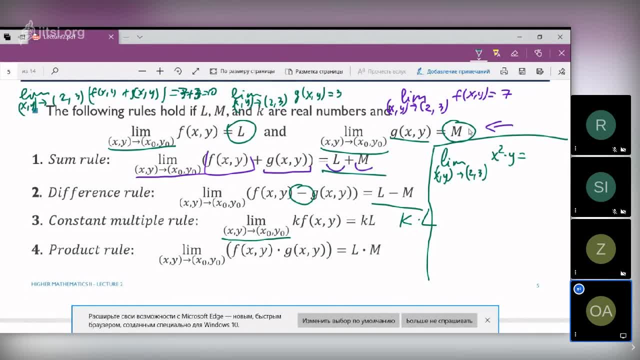 it's a x squared. x squared is number two. we have to, so two squared times instead of y. sweet, okay, is three times two. 4 times 3 is 12,, right, 12.. Is this clear? Okay, Now, according to the conflict, multiple rule. 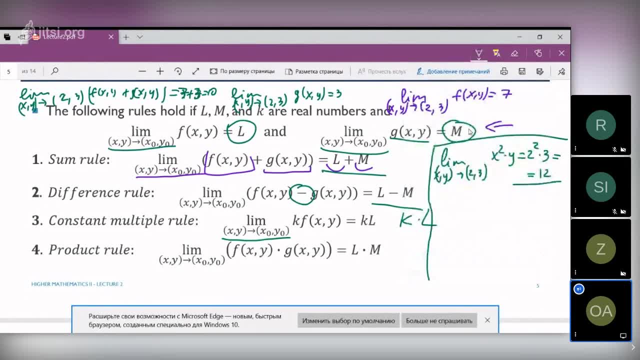 Yes, yes, circle. in this case, we may have this kind of example: We need x and y times 2,, 2 and 3, and 13 times x squared y. Can you calculate this? Yes, Sure, Okay. 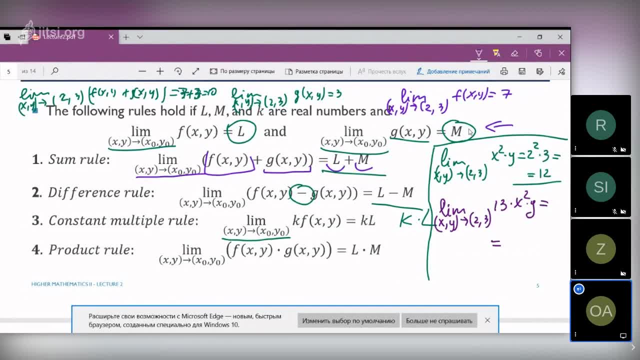 If you do it there, okay. According to the circle, which is constant multiple, I have to write 13 times and then I have to calculate the limit, which is x squared y, when x, y tends to 2 and 3.. 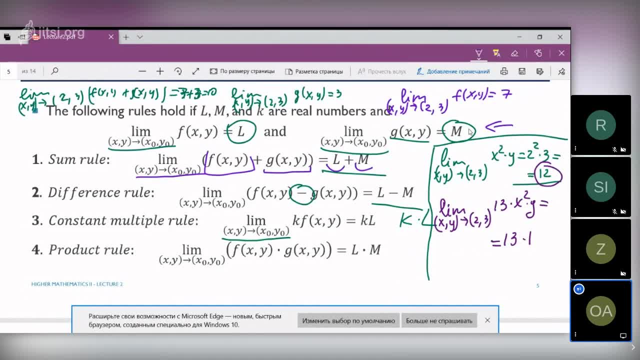 But I already I have 12.. It's 12.. Like this, So 12 times 12. It will be how much 144.. 144 plus 12.. 154.. 154,, yeah, 156.. 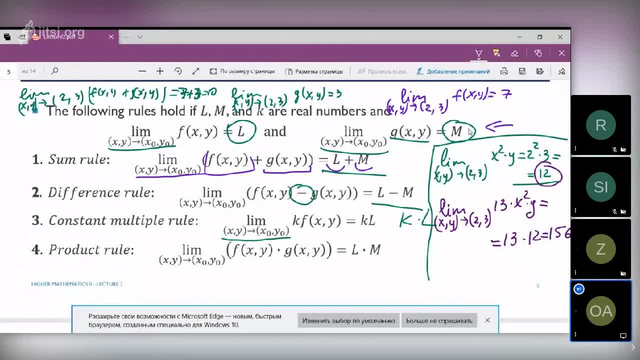 So 56.. Because 12 times 12 is 144, and plus one more 12, it's 156.. Yes, Yes, yes, yes, 156.. Okay, This, I've calculated this one using the circle. 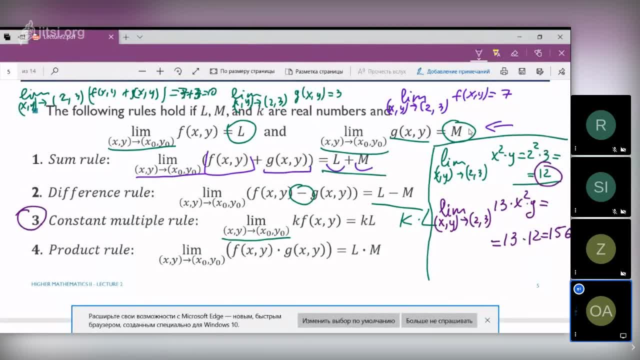 which is constant multiple, And in the fourth. in the fourth one, which is product rule. it's similar. Thank you, Instead of this 13,, I will have another function, another function, And I have to multiply both of them together. 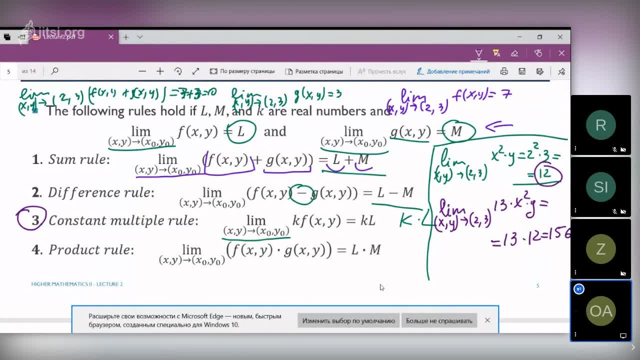 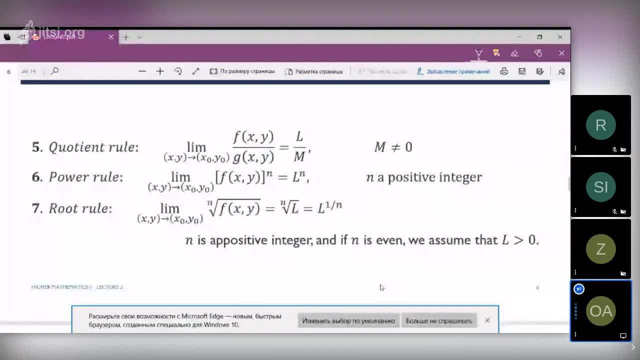 I will get the final limit. Thank you, Okay. Thank you so much. Thank you, It's adeath of love. Mm. hmm, We have some more rules: Quotient, we'll take more. Okay, It's the quotient rule. 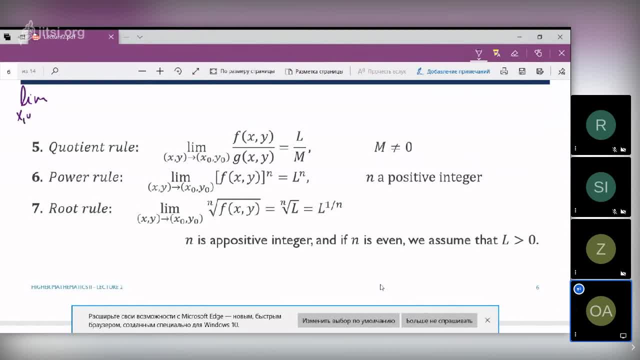 Mm, hmm, What's our example? Limit xy times two, 1 and 3, x squared y. again Again, how much. this one, Three. This one is one, second, one is two. One, one, one, two and three. 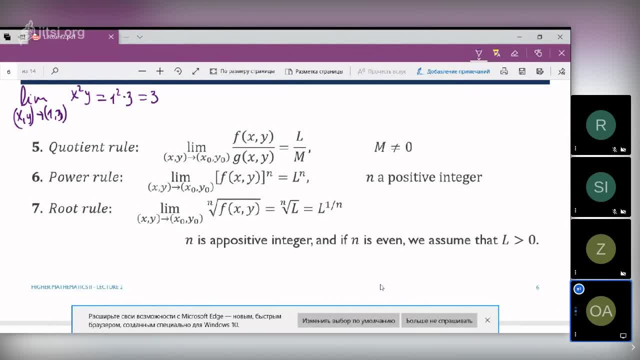 Answer is three. Yeah, All right, You guys know the number here. you did it. Next slide One, two, one and three. again, We have to find another. It's also three. yes, it's also three. 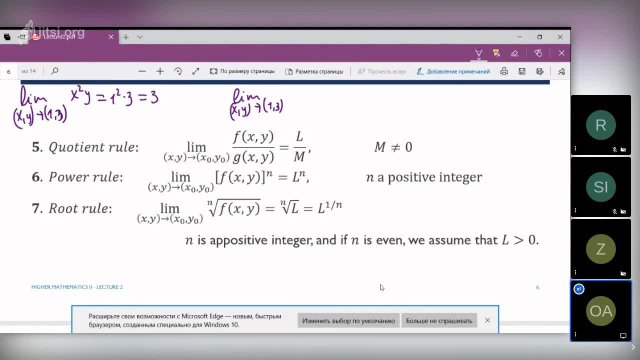 And the general answer is one: The function is a fortune. No, no, I didn't wrote the function yet. okay, Mm-hmm, X cubed, y cubed, Yes, So X cubed, which is one. 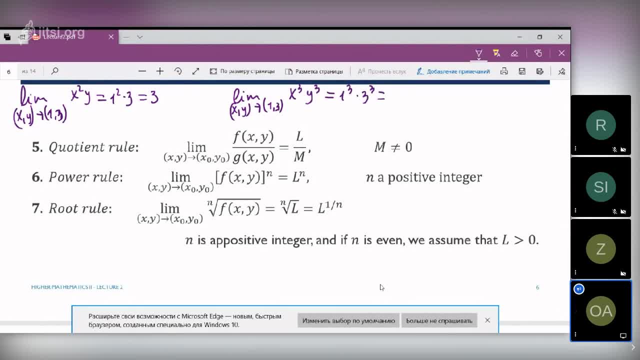 y cubed times like this: three, two. So the answer is one, two, three, one It's nine, 27,. maybe It's nine, Ah, 27?, Yeah, 27.. Ah, yeah, yeah, yeah. 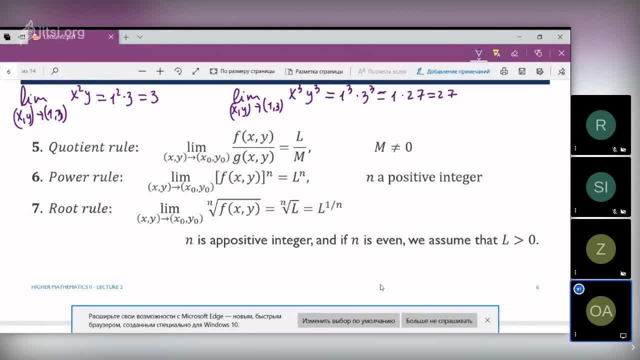 Just this one, 27.. 27.. Now you have to use quotient rule for the next example. For example, I want to write here: limit X Y times two, one and three, And I have quotient here. 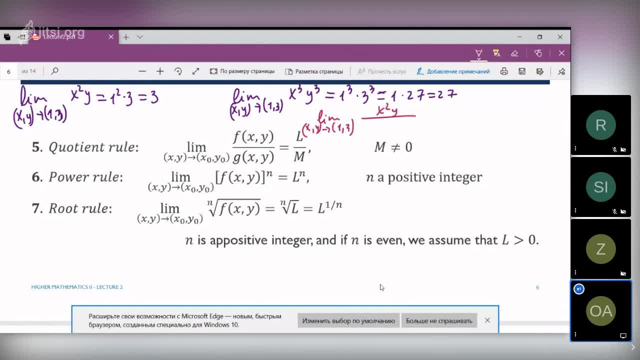 Upper part is X squared Y and the denominator X cubed times Y cubed. We have two ways to calculate this. one here It's a search over 27.. First of all, if you use the answer, then you can simplify this. 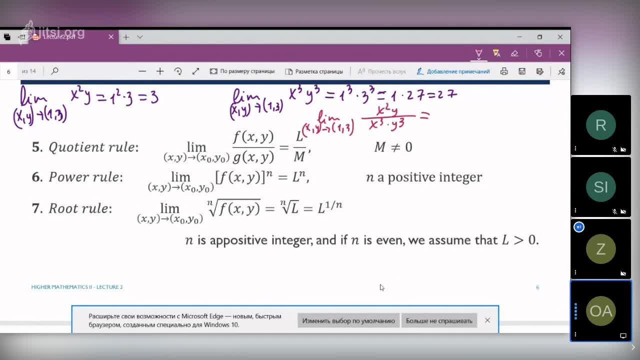 You can think about it if you want, but if you don't want to simplify, or it's hard to simplify, just use the quotient rule, which is given with one five. Do we know the limit of f, of X, Y, which is this one? 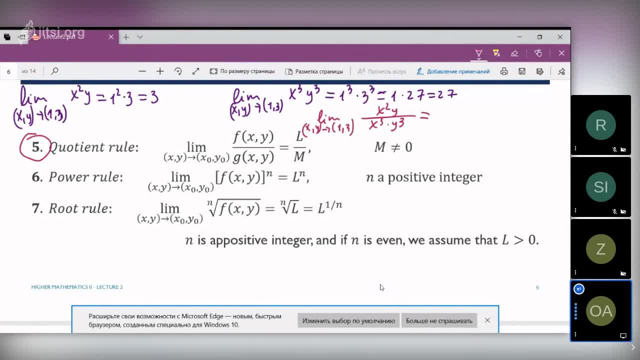 We have to know The limit of the numerator X squared Y. five is three- just now we've calculated- and the limit of the denominator Y is Three, yeah And 27.. Yeah, that's right. 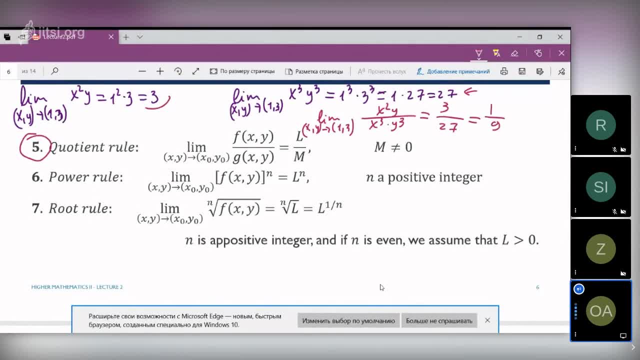 Now we can simplify this. It will give us one over nine, One over nine. One over nine. Yeah, it's one over nine. This exercise we've calculated using quotient rule, which is given with number five. I'll tell you that you have to be careful. 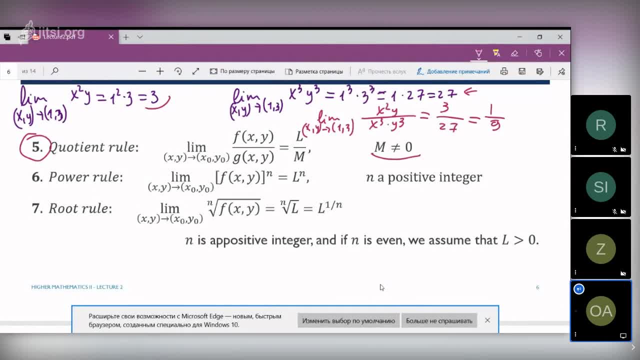 while doing this rule that the M should not be zero, M should not be equal to zero. Yes, yes, yes, Because in the denominator we cannot divide by zero. Uh-huh, Because at this F it should not be zero. 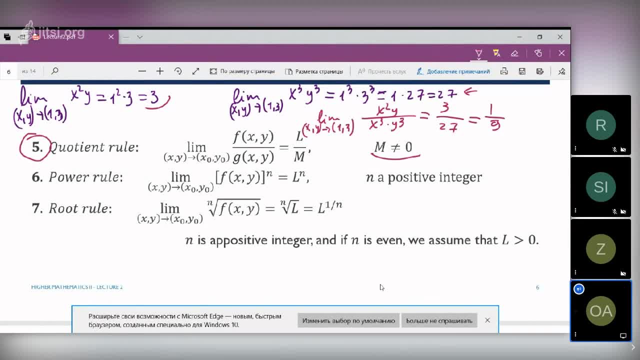 Pay attention to that while solving exercises. We have to- yeah, we have to- simplify this one, yeah, Yeah, if we have this kind of expression, we have to simplify or like, try to rationalize. if it's irrational, try to rationalize. 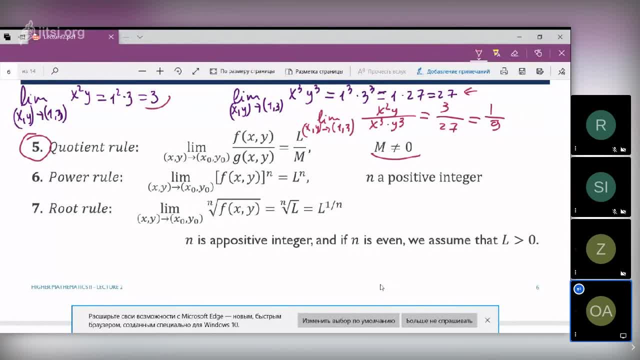 and then we can fix it. Yes, yes, We can find its limit. Okay. the next one is power rule. Power rule Limit. X Y tends to X. zero Y, zero F of X Y's ends power. 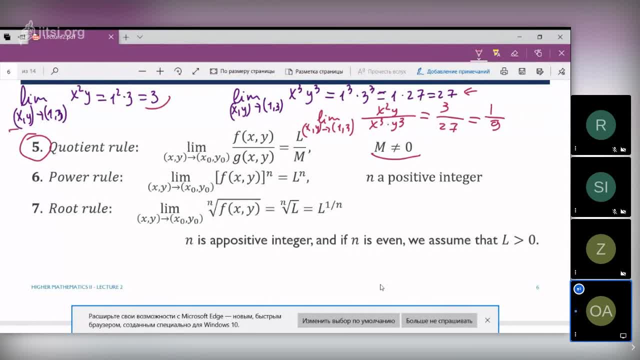 Good limit will be L's ends power. Now we have this expression, The first, For example. I'll try to use that one: Limit X- Y. It's comma Tends to one and three X squared Y, And this one will be limit X- Y. 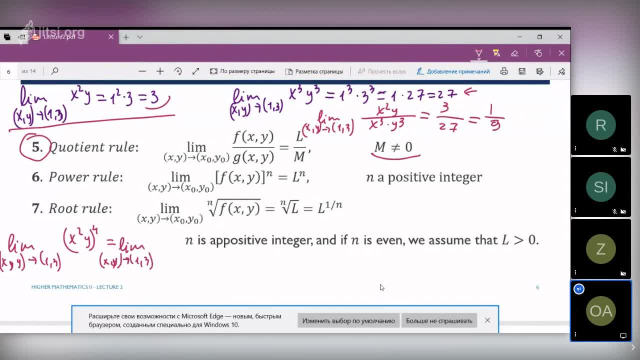 Tends to one and three And X. X squared two times four is eight times Y to the fourth. You can calculate this one by plugging in numbers One instead of X and three instead of Y, Or you can use this rule. 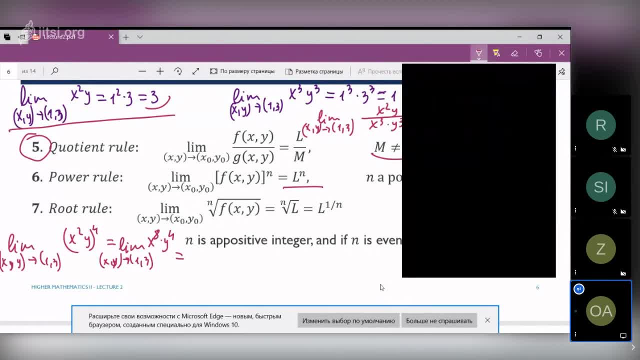 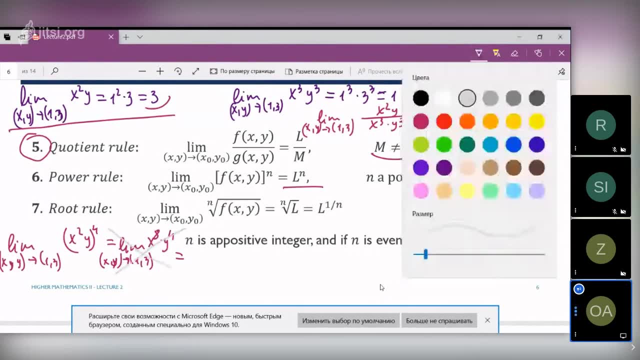 You can use this rule also Without this one. If you use that rule, you will not need this. You will not need this one. If you use the rule, you have to write your. you know the limit. it's three. so the answer is three. 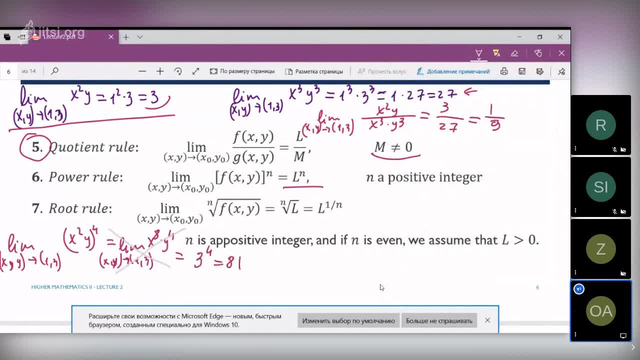 Three to the fourth, 81.. But you also can use, by finding its power, X to the eight and Y to the four, and plugging in one here and two here. The answer remains the same. It depends to the situation which you are solving. the example right. 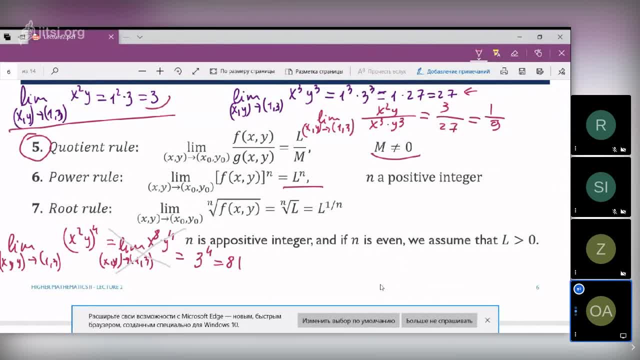 You have to look through the example and find which is the better way, Which is the better way, Which is better to calculate. And finally, rule number seven: root rule. Root rule. Root rule In this class: Yeah, Root. 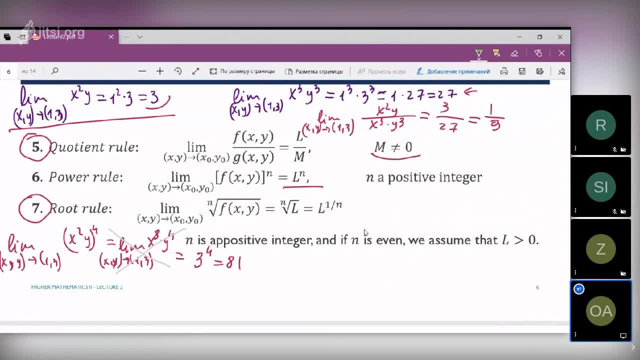 It's similar with the power rule. In the power rule we have the number here. In the root rule you have number here. Yeah, So we have limit X, Y, points X, zero, Y, zero And the function f of X, Y under the root with M's power. 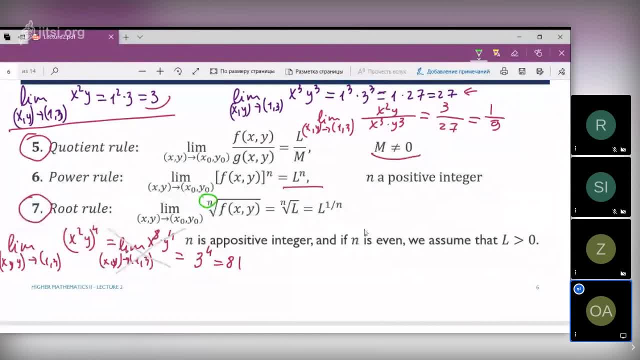 So we can. if we know the limit of f, of X, Y, we can write this one And from this I can write one over M. Both are same, both have M, But pay attention, we have both. M is a positive. no, there is extra P. 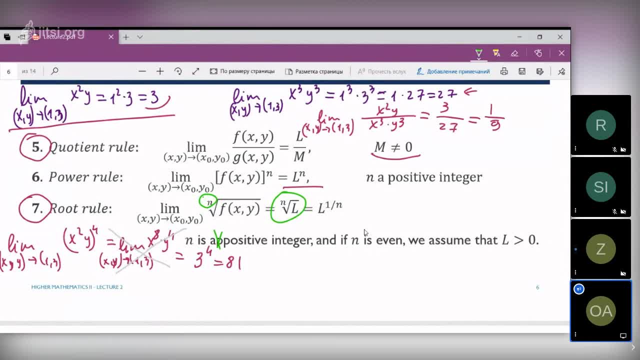 M is a positive integer, Mm-hmm. And if M is given, we assume that L is positive, Because we cannot find the negative numbers square root. If M is, for example, if M is number three. Yes, yes, yes. 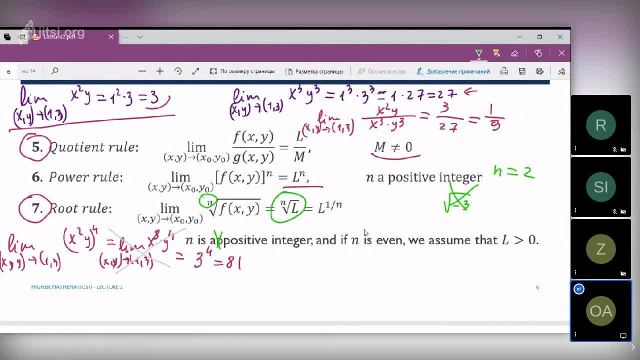 We would have here. so minus three, So we don't know this one. Or if M is number four, four is equal to minus 16.. So we don't know this one. It's not defined. But if M is number three, it's okay to have a third root of negative 27.. 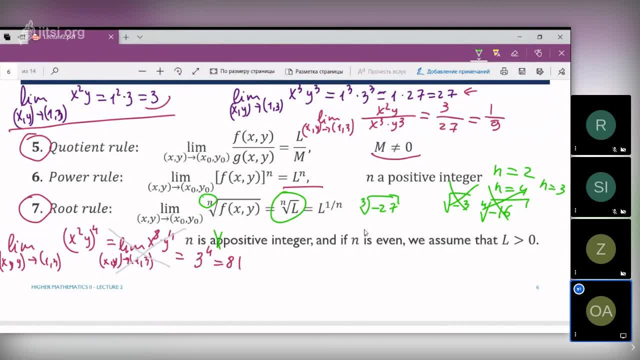 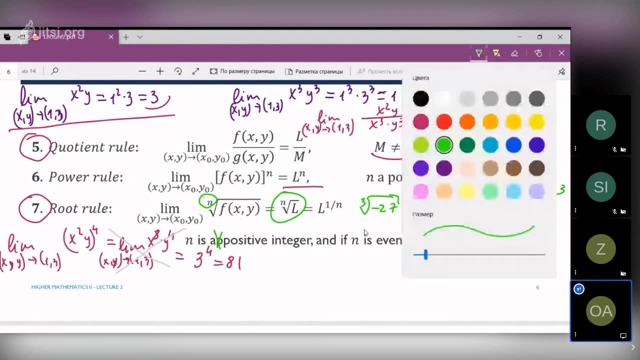 It's okay, But when M is, even when M is, even again, just watch it. Let me give you an answer: Mm-hmm, Mm-hmm, Mm-hmm, Mm-hmm. 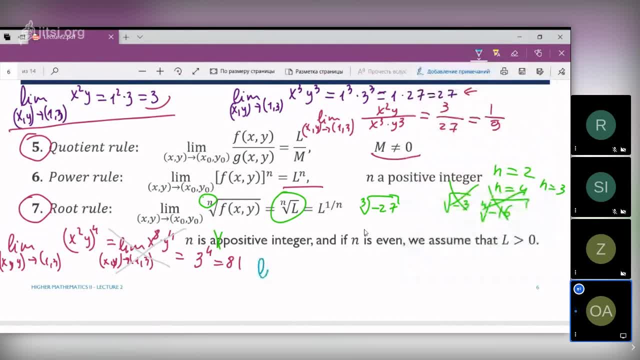 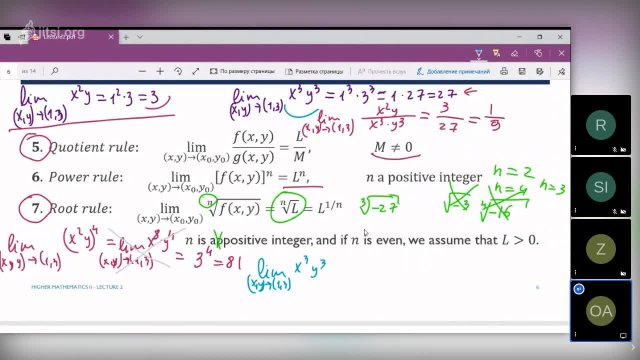 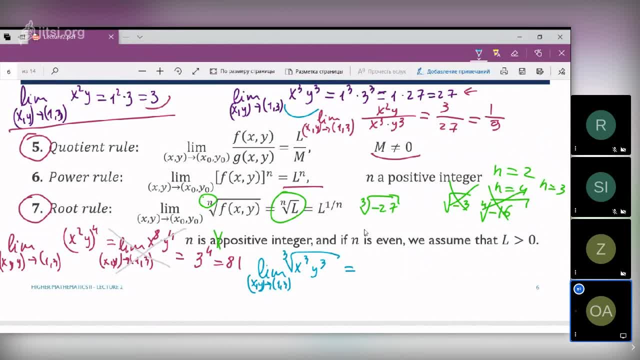 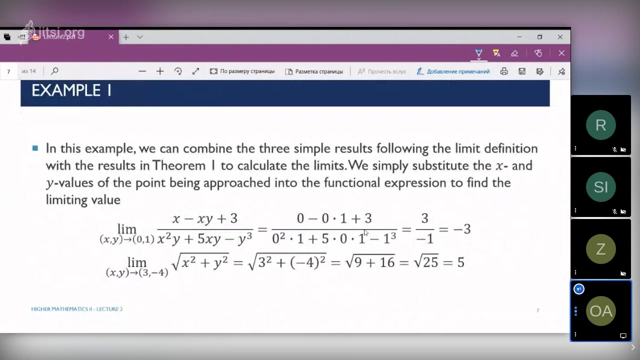 X cube by Q under third root. Okay Require to. We know how to calculate. We know the limit of this expression. It was 27.. So Q root of 27.. In this example we can combine the three simple results following the limit definition. 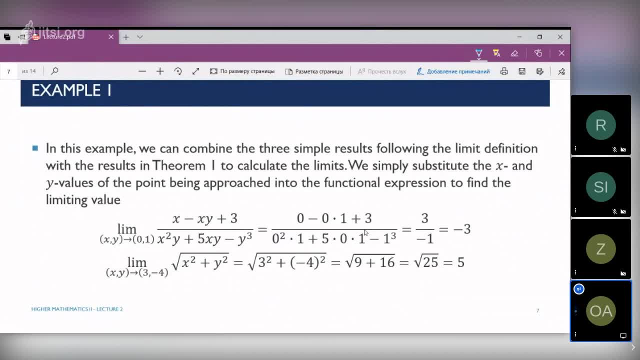 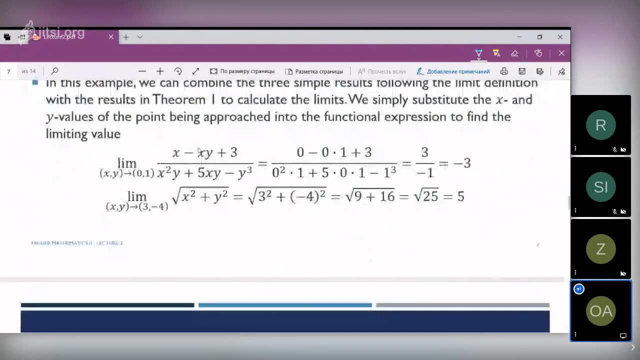 with the results of theorem 1 to calculate the limits. The simple substitute with the x and y values of the point being approached into the functional expression to find the limiting y. This is a little bit big example. It's not terrible, It's super easy. 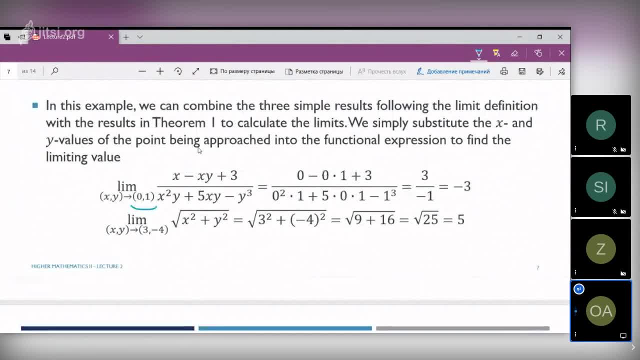 It says: limit: x and y is 0 and 1.. And the function is this one. How cool is this? You see, the x wasn't 0.. You see the y wasn't 1.. The x here is 0.. And x 0 here is 0. 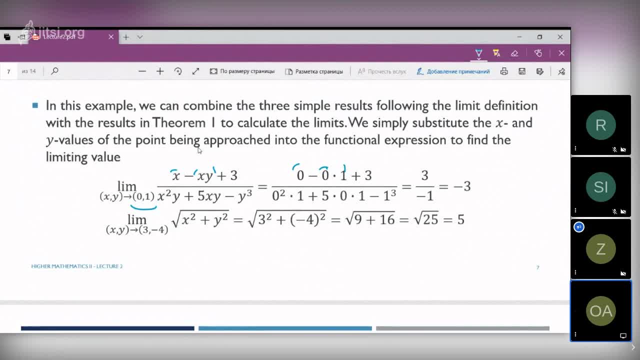 The y here is 1.. That's the result. The x here is 0.. The x here is 1.. The y here is 1.. 5.. 5 is the result. It's constant after it. 30 is the constant after it. 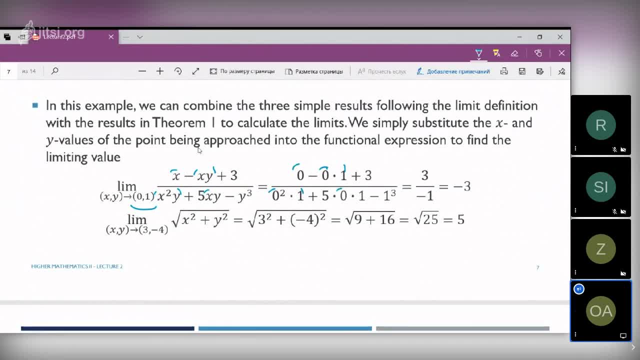 3. 0.. 0.. 3. 1. 3. 1. 2. 1. 1. 1.. T d p 0.. 1. 0.. the next example says limit x, y tends to three and negative four. so it says x tends to three. 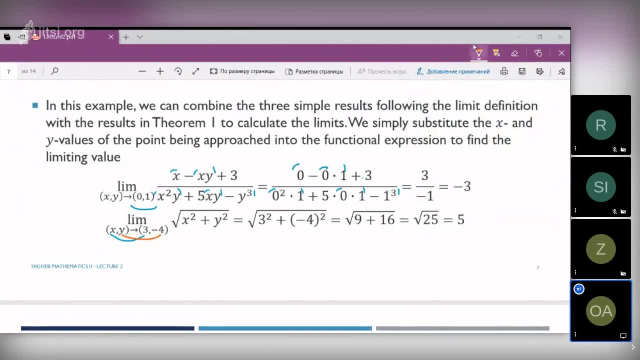 and the y tends to negative four. oh yeah, so the function is square root of x squared plus y squared x squared x is three, so it's squared plus y squared negative four squared three, squared nine plus negative four squared is sixteen. nine plus sixteen gives us twenty five, square root of twenty five. 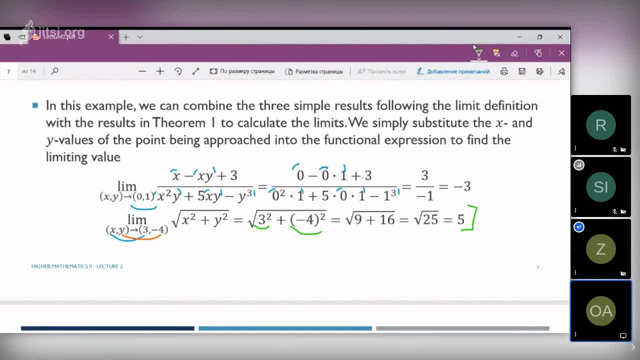 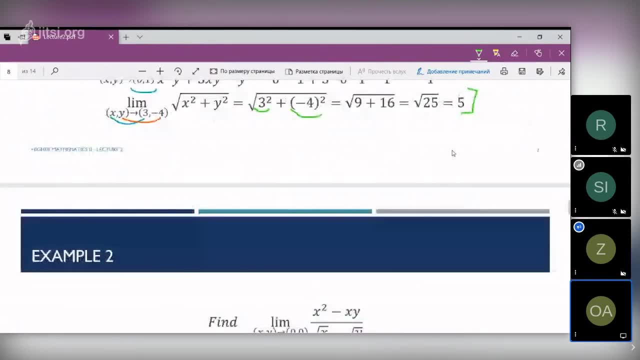 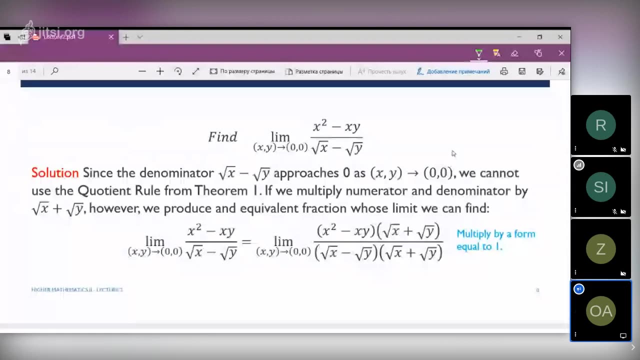 it's five, it's five, yeah. yeah, we have done with this first example. and the second example says: find limit when x and y tends to zero. if we plug in instead of x zero and instead of y this zero, i will go here: zero minus zero, squared minus zero times zero. 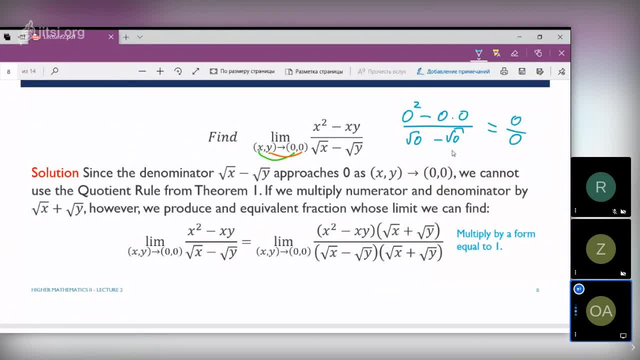 yes, it will be zero over zero. yeah, it's undefined. yes, so we can't solve this one, since the denominator square root of x minus the square root of y approach zero. as x, y tends to zero, we cannot use the quotient rule from. we can't use this. 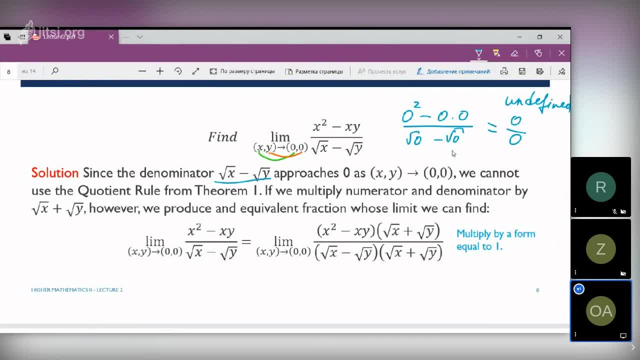 first of all, we have to simplify our rationalize. if we multiply the numerator and denominator square root of x plus square root of y, however, produce an equivalent fraction whose limit we can can find. okay, try to multiply by this expression, so the upper part will be x squared minus x y. 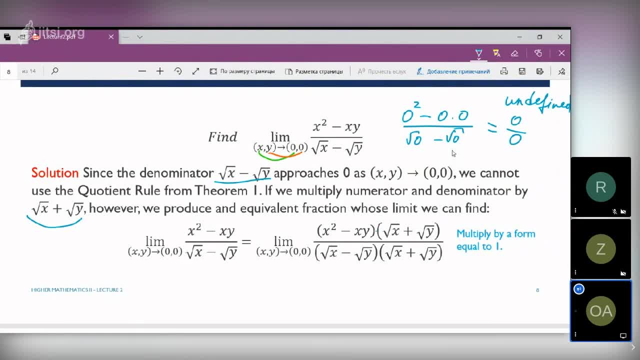 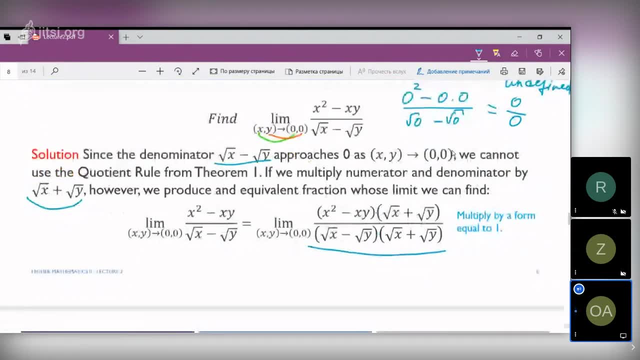 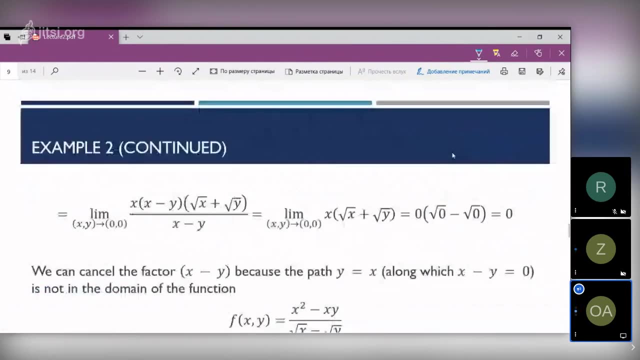 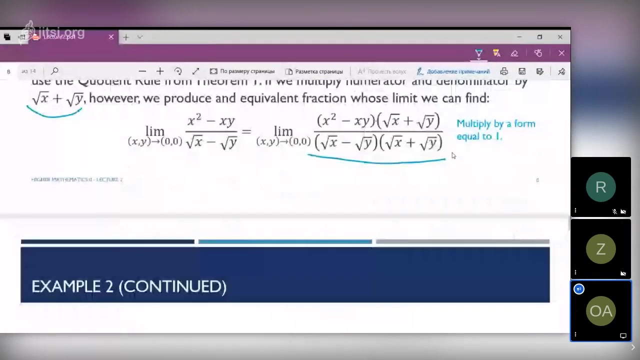 times and the periphery is square root of x plus square root of y. in this part also, this expression, this new expression, gives us x minus y and in this part also to open. if you open the pair into this, you will get this expression not open. if we take these things outside of the kind of yes, if you take this. 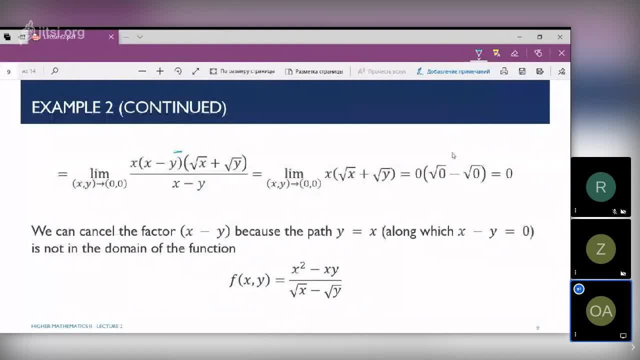 out of the pair to this, we'll get this expression. okay, so they are done. it's minus one x minus one x times two x plus square root of one. now we can put zero because the zero one is constant. we can't cancel because via the zero 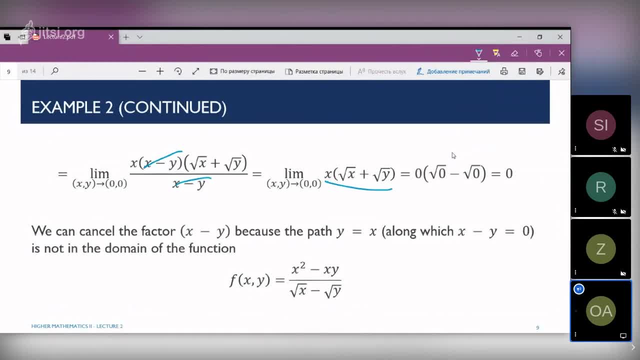 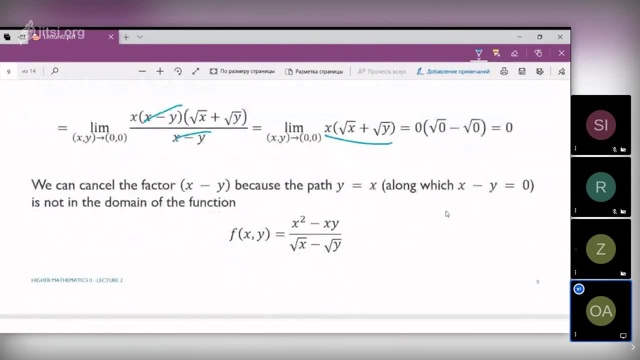 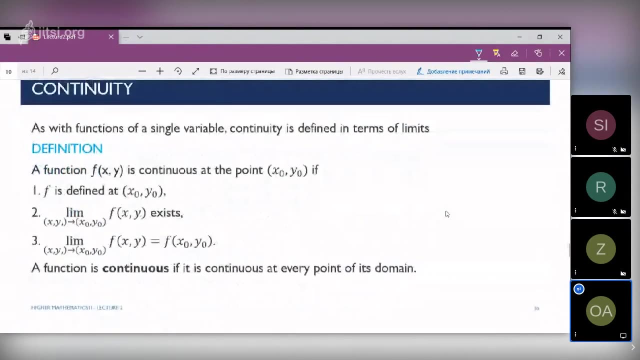 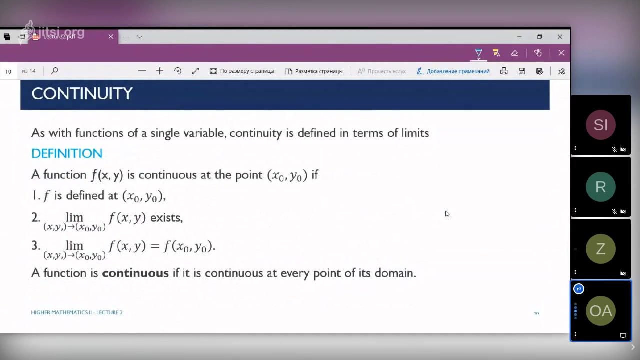 it's not in the domain, so it's easy to cancel this expression. as i said before, it's similar to functions of az single variable to calculate their limits. now let's speak some words about the continuity. we're almost done with limits of several variables. we understand the concept. how to calculate some limits? 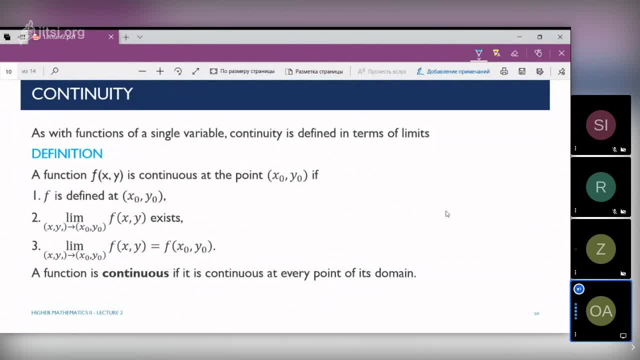 um, how to do? what is that now about the continuity? as with functions of single variable, we have three rules, three steps to check the continuity. the definition says the function f of x y, f of x- y is continuous at the point x- zero, y zero, if first one f is defined at x 0 y 0, f is defined at x 0 y- 0. for example, f of x- y equals to x over y. 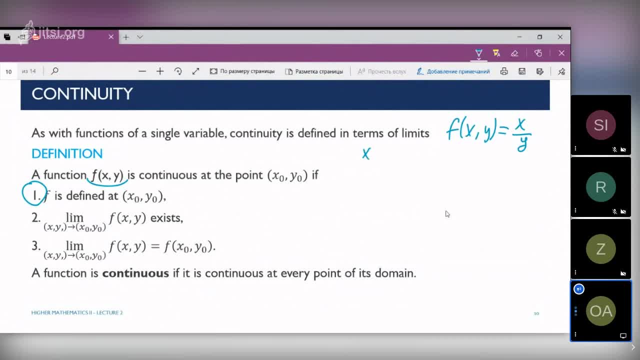 for example, this is a function and x 0 y 0 is. x 0 y 0 is like one and zero. the first rule says f is defined at x 0 y 0. if i put one and zero here, i will get one over zero. 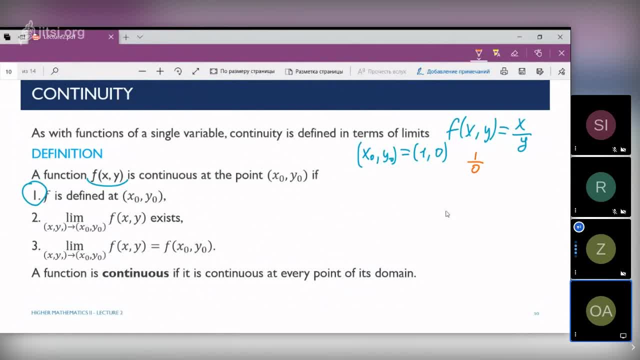 so is it possible to divide one by zero? it's undefined, yeah, yeah, it's undefined, so it's not defined. the first rule, it failed. first rule fails. so this first rule says about this one. this rule says about this one. if it's not like this, if we calculate this one, the first rule will be acceptable and we will move to. 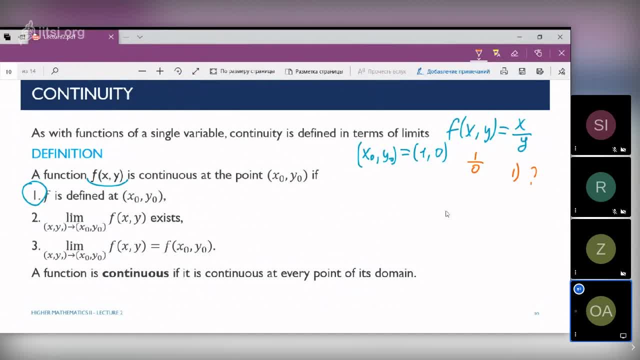 the next one limit: x- y tends to x zero, y zero. yes, f of x- y exists, f of x- y exists. And then we'll move to calculate this limit When it stands to one and zero: x over y, So one, it will be one by zero. 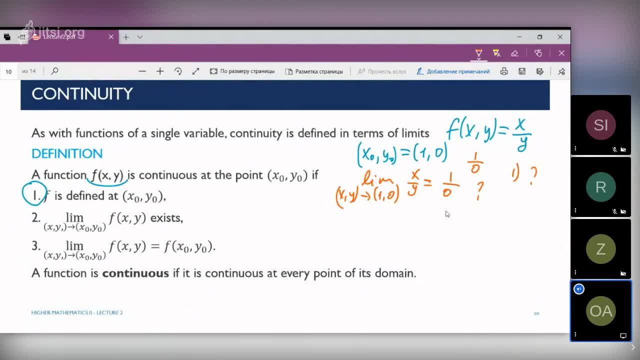 And it's also on the five. We can calculate, we can divide one by zero. And the third one: this limit's value and the value of the function must be equal to each other. They must be equal to each other. Only in that case we can say the function is continuous. 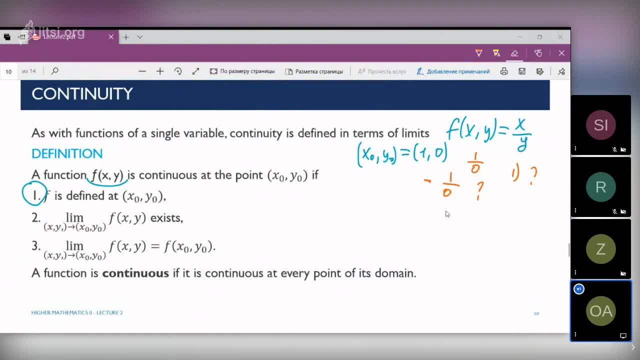 at that point. For example, we can check this function at another point, Not the zero. Let us choose other point: One and three. So the value of the function f of one and three equals to one over three. Then limit when x and y. 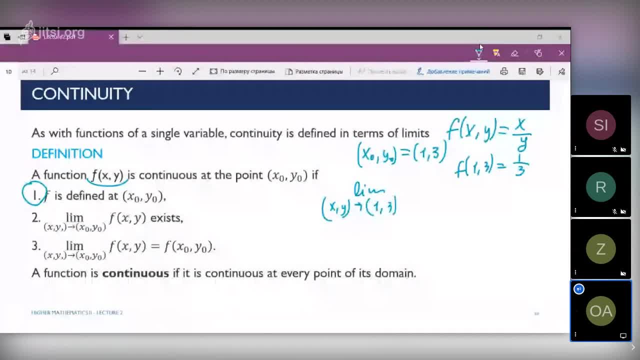 It's possible. one and three. x over y is one over three. There it's also calculable. The third rule says this: together should be equal to each other: The value of function and the value of the limit. Are they equal to each other? 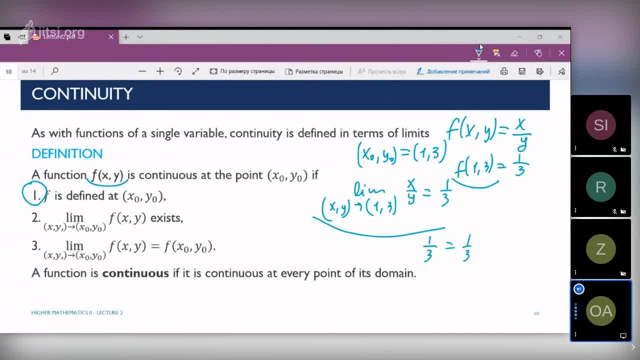 Yes, one over three equals to one over three. So we can say: function f of x, y, which is x over y, is continuous at at one and three points. At point one and three We can say this one, Because we just did this. 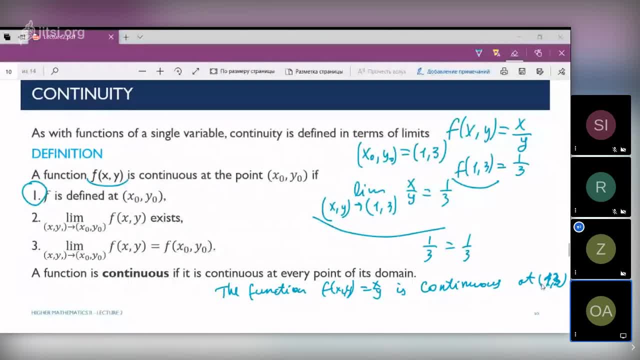 Check this. That's right there At point one. Remember at what point. What's that? At point one, three, One: If you have these kinds of similar questions or exercises in the book or in a homework assignment, check the function of continuity at this point. 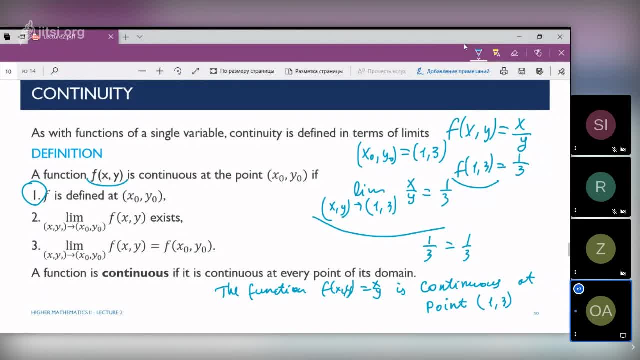 You have to check like this, Step by step, And the right answer is both: The function is continuous. It is continuous at every point of this formula. So this one is, We can say the function of continuity is continuous at every point of this formula. 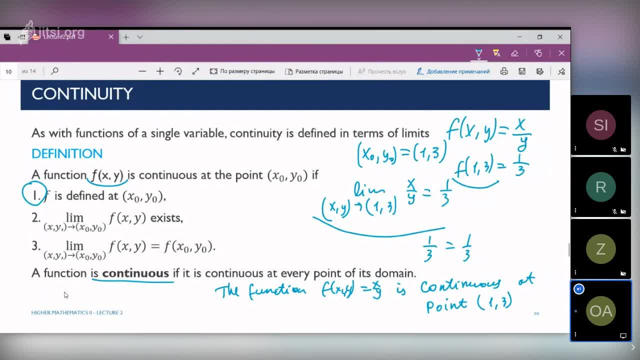 Just now, we set the function of continuity at one point. One and three, Just one point. The function of continuity at every point is the one that's going to be selected. So we can call the function of continuity One, One, One. 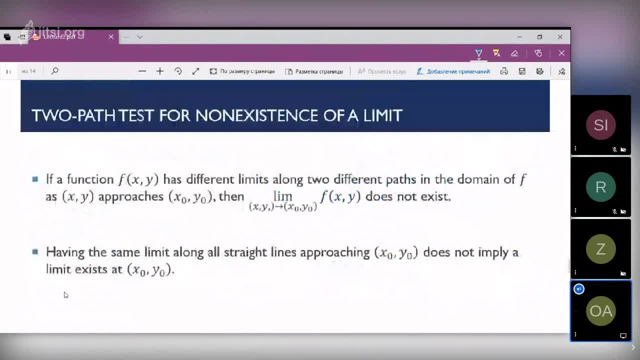 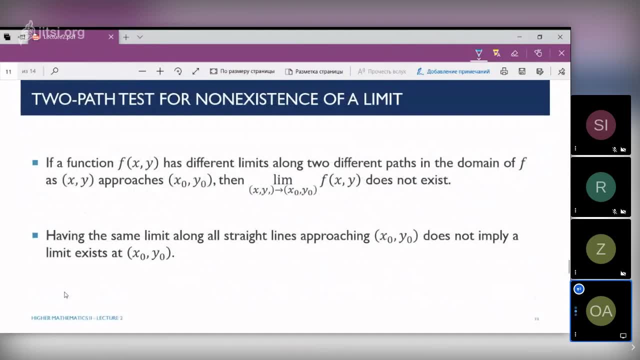 One One, One point One, two, three, four. It's comming from one point, One point, One point, So we're going to have some. We've got two types of paths for non-existence of the limit. 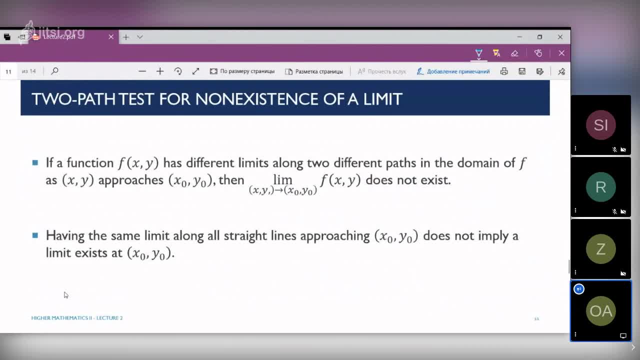 And the function of spacey has two different paths. So I have three different paths. The boundary I have x1, 2, 3, 0, 1, 0.. Then mu: x1,, 2,, 3, 1, 0,. 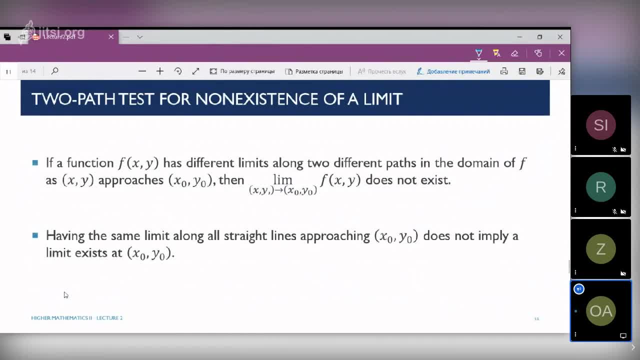 and this is another, And the right answer is two: Having the same number of holes throughout the portion of the x-ray laser. we have required a limit of the x-ray laser. It is similar to the right side limit, to the left side limit. 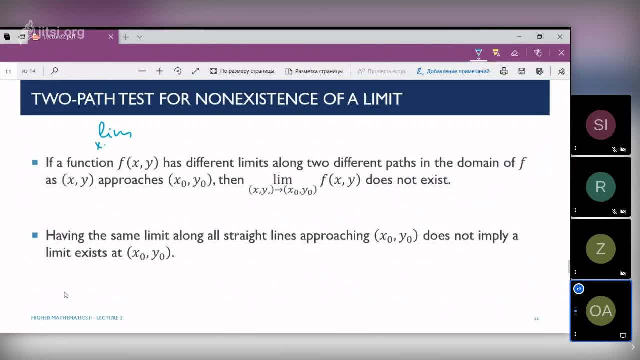 If you have a look at the limits of the limit, x goes to 3 from the left side. x-ray limits are limited. x goes to 3 from the right side, x goes to 3 from the left side. if you remember, we had these numbers expressed for the function of two layers: right side limit and left side limit. 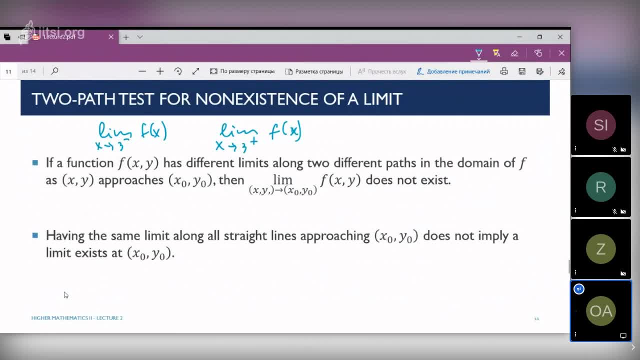 For the function of several layers, especially for the function of two layers, we also have these types of limitations. So the function of x1 has two different limits for two different types, and the dominant one has a different concept here. and the dominant one has a different concept here. 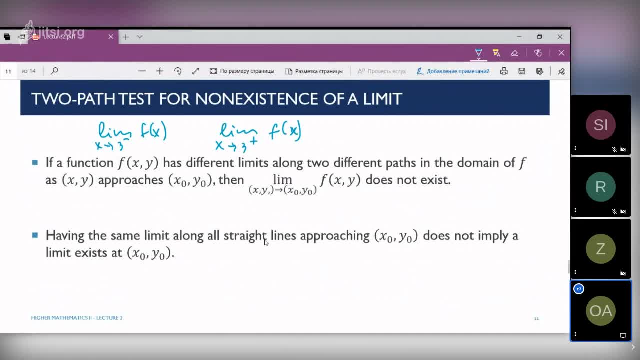 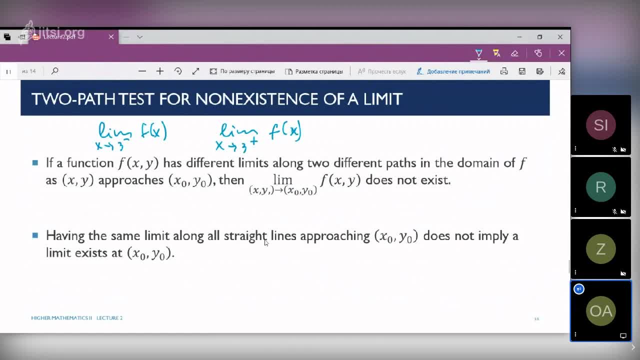 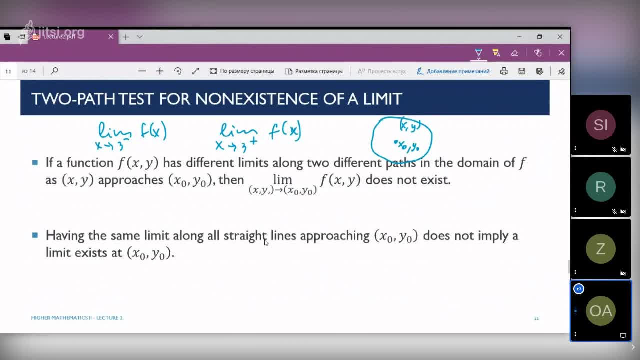 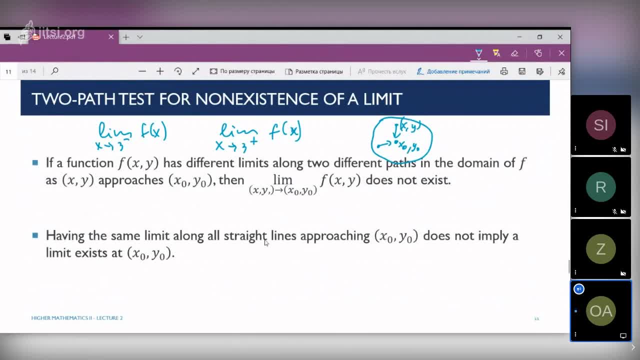 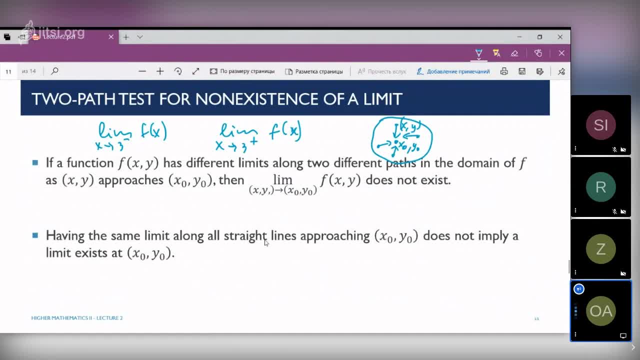 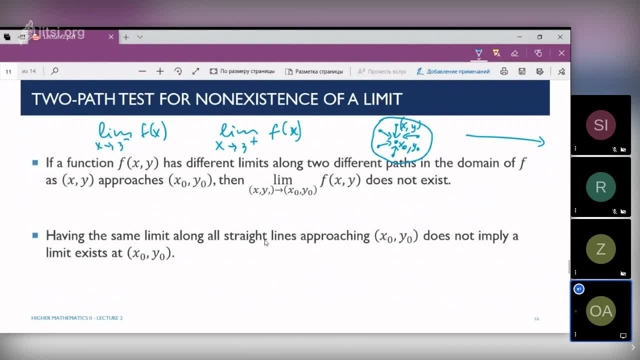 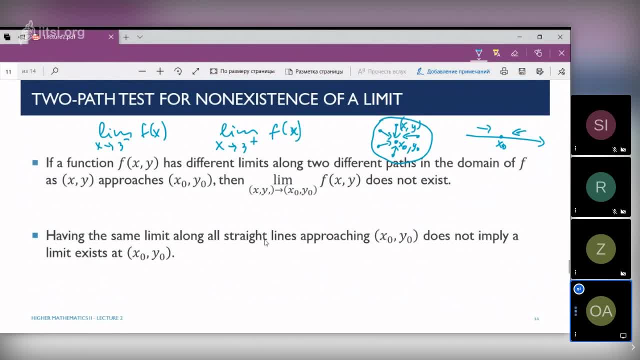 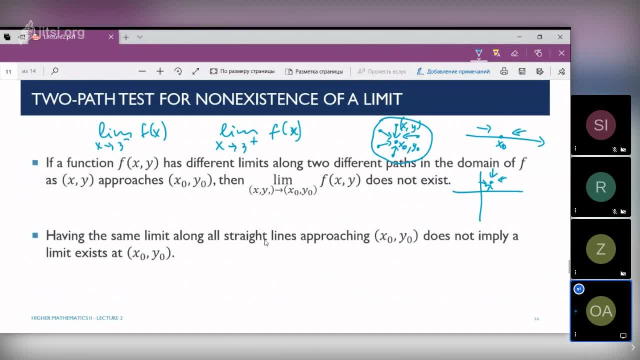 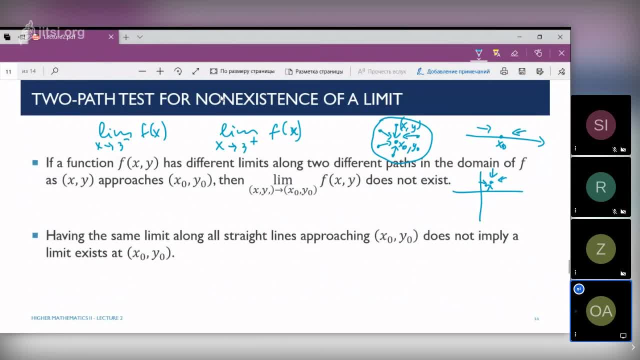 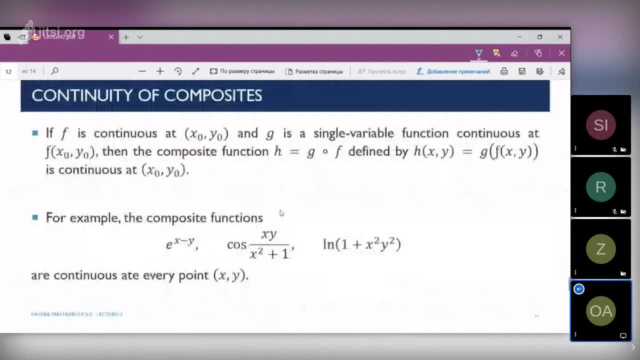 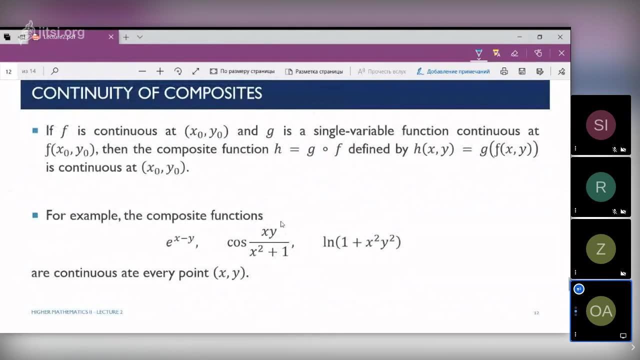 This is how it works: Continuity of components if F is continuous at X0, Y0, and G is a three-level component continuous at X0, Y0.. The composite function is G, composed of X defined by F of X- Y, G of F of X- Y. 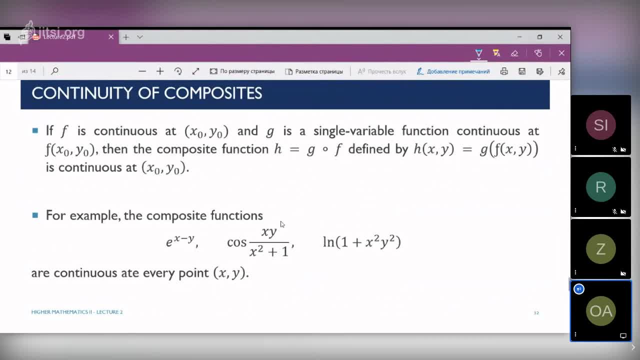 It's continuous at X0, Y0.. We also learn the composite functions. If you remember, we learned composite functions and I have made one. Some of you, some students, read this now as GOAT right GOAT. 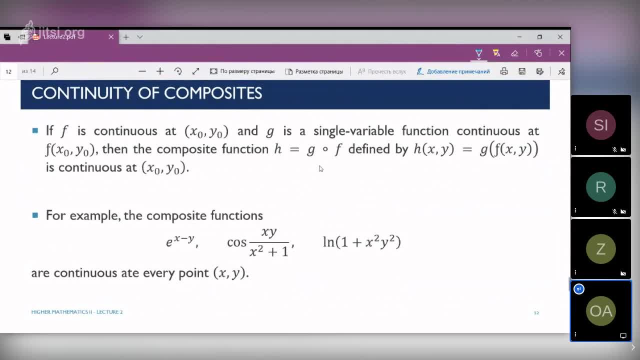 It wasn't GOAT. it's a composite function: G composed by F. What does it do? Since I did this, things have been a whole lot better. It's easier to do than happening. it's easier to do than writing. 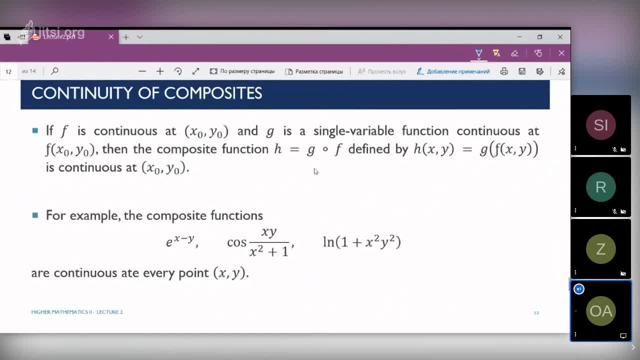 It's easier to do than fiction. you know We have done a lot of scary things. for example, That's what I'm doing. You know it's not just a normal thing. for example, Within the first function we have X0, Y0, Y0, and G, and G is a three-level component. 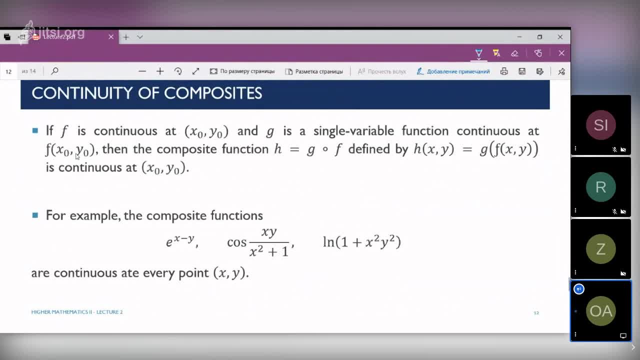 Instead of X0 and Y0, Y0, Y0, and G, we have a three-level component. Now we see a part of the function, a non-functional function. The function that we have is the function that we have to write. 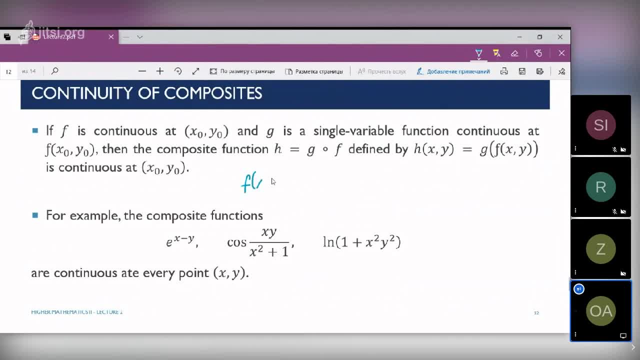 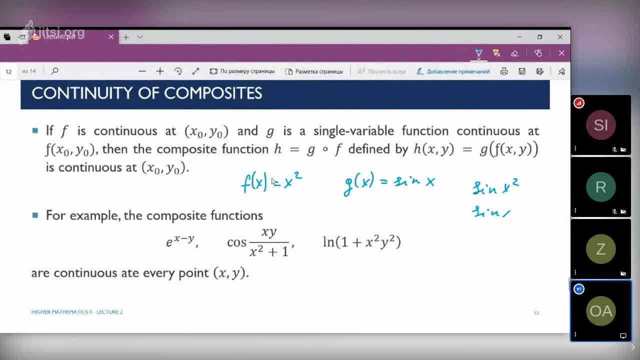 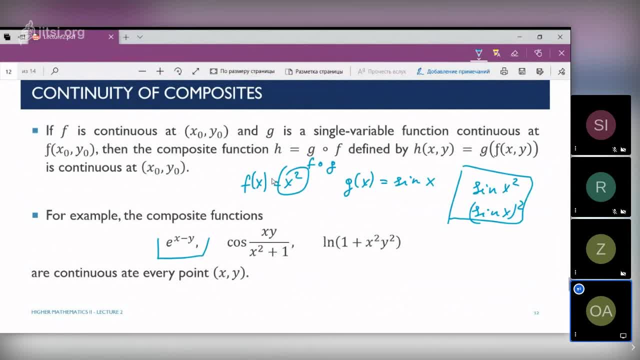 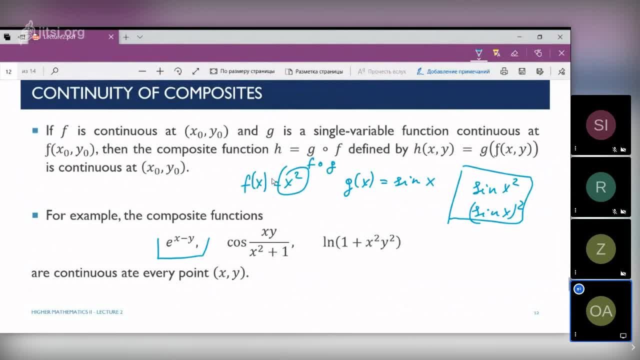 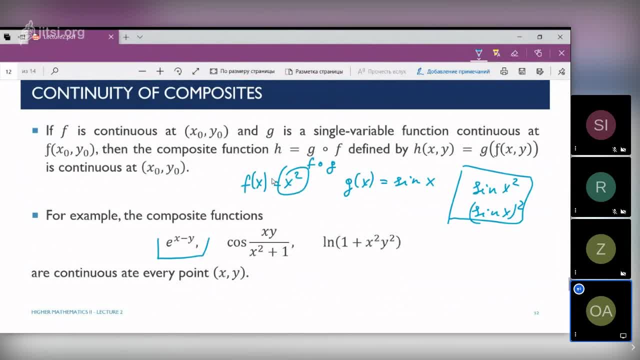 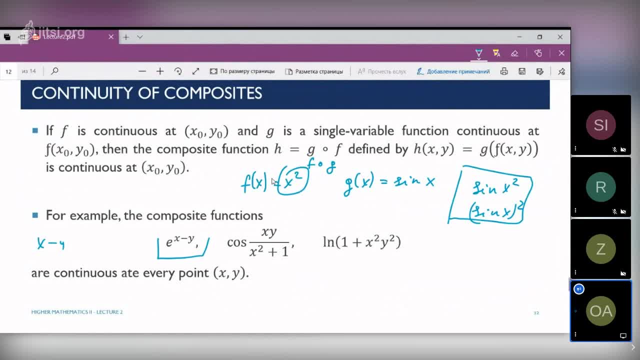 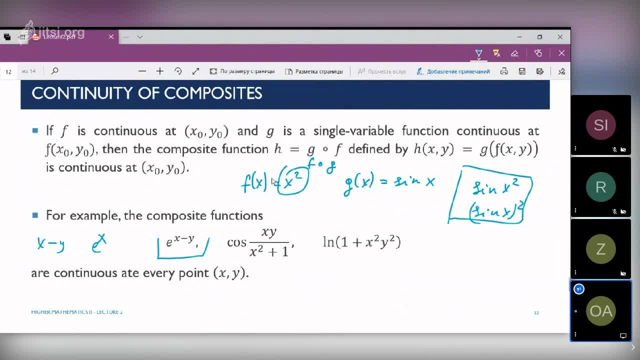 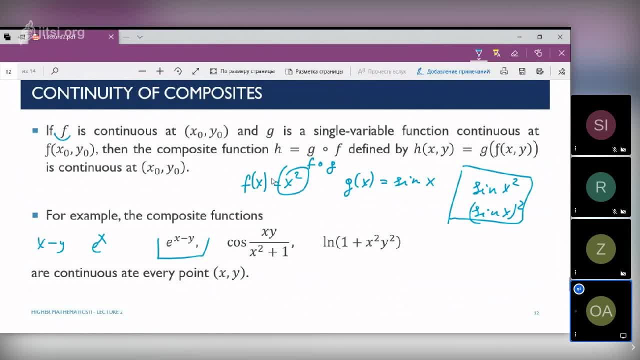 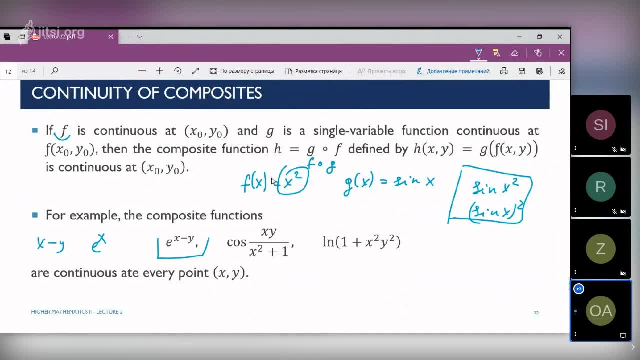 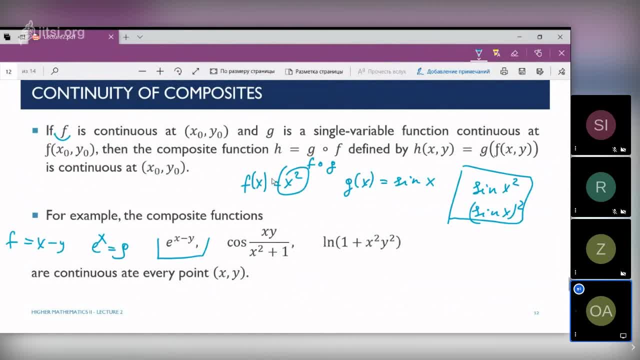 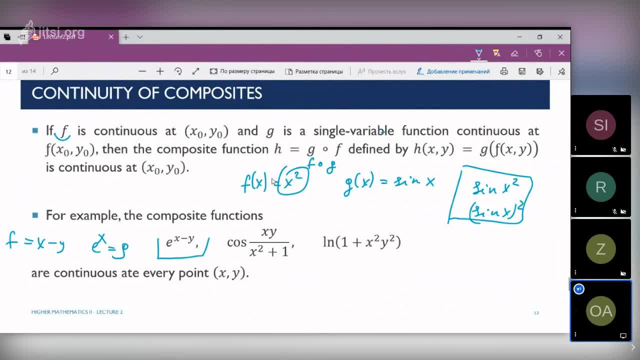 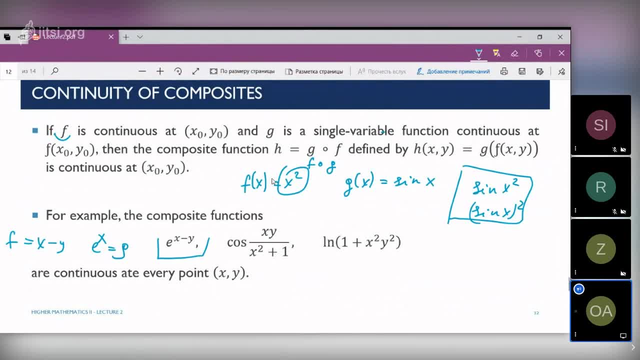 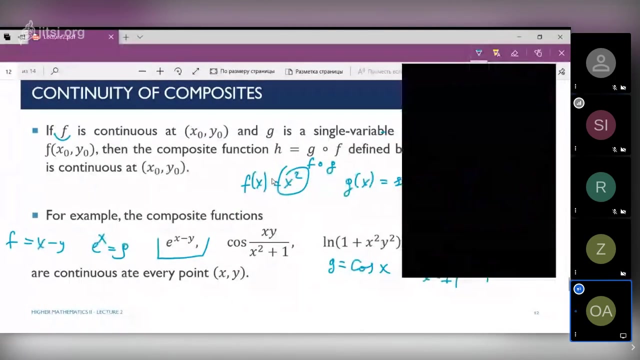 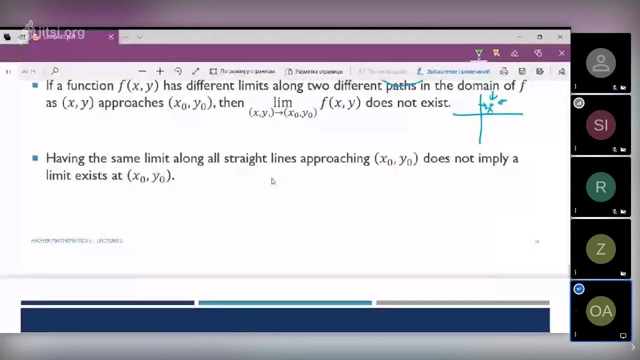 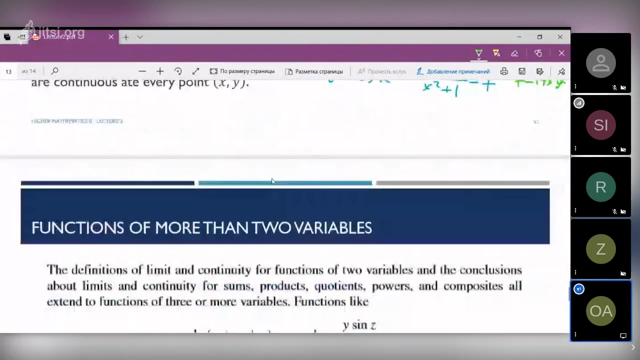 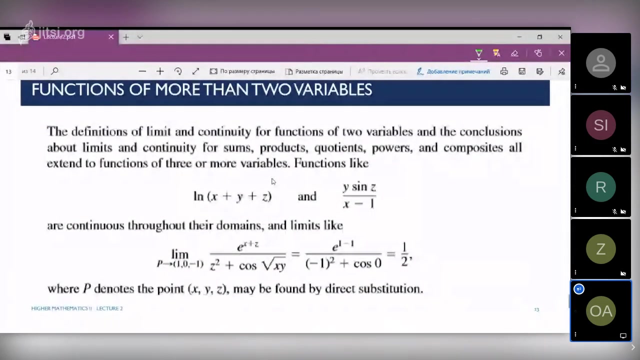 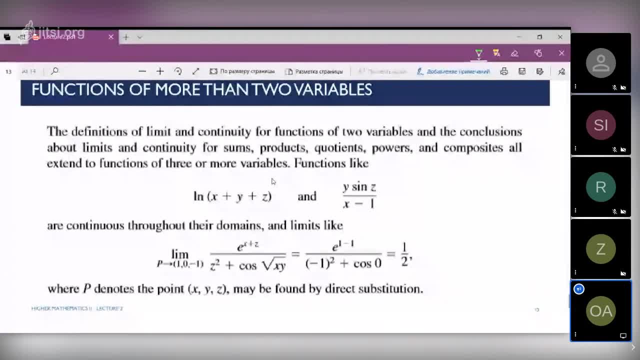 Two rows, Four rows, Three rows, Four rows. In that oils and has Th At Th At And rest of OEMS. Okay, Thank you, It is Okay, Thank you, adjust, Okay, Let me, It's OK. 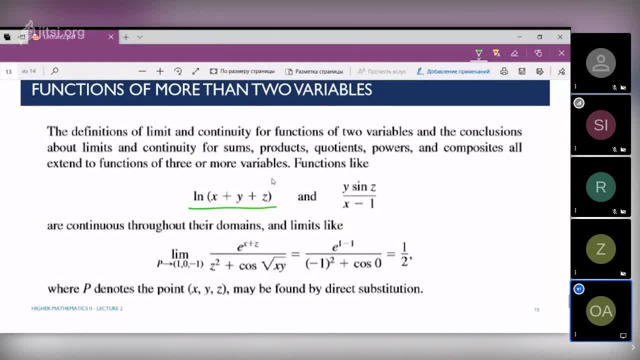 No, Just do it right There, There. All right, That's it. Okay, I have one row. I have ven. Let me fix it. All right. Then it is D. I think you have Right, All right. 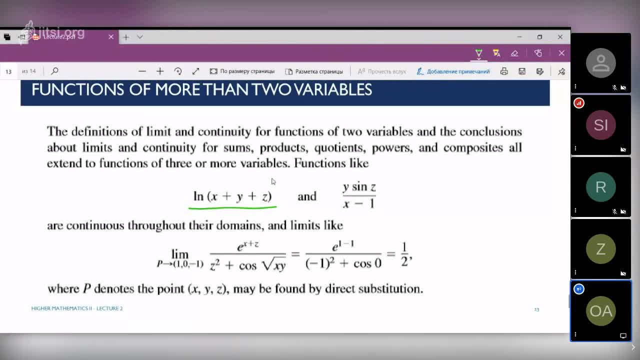 one, zero, negative one. so this is a sequence: one- this one is zero, is y and this negative one. what is that? you have to try to understand this one here is negative, one negative one, one and zero, and we have to calculate this expression if we have function of three. 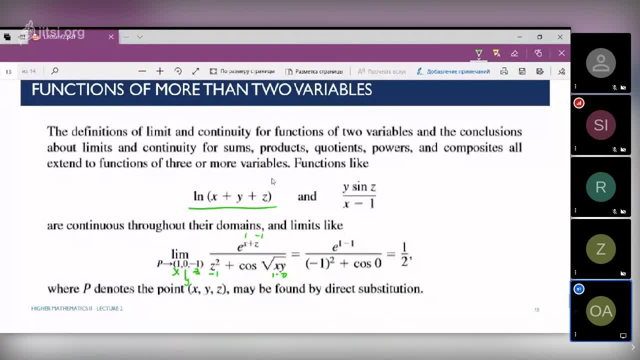 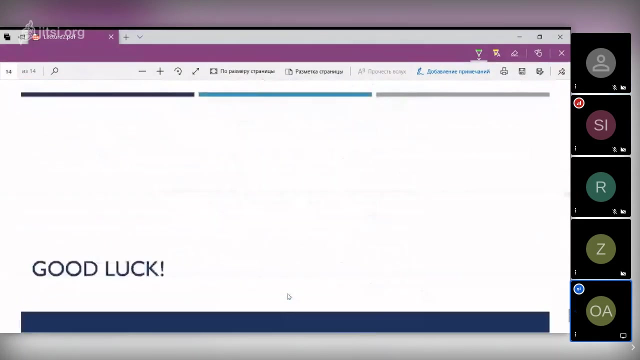 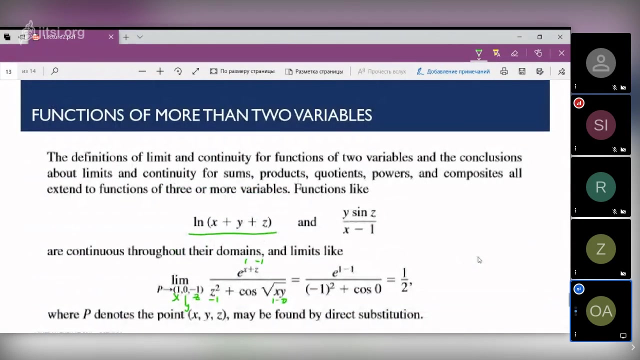 oh, is foreign foreign. so this is the. this is the part of the function of three variables and their units and we're going to have the top five. there are a lot of possibilities. examples before for you guys. if you are clear with this theory, you can solve the exercise and we'll continue our steps after a break. now you may.